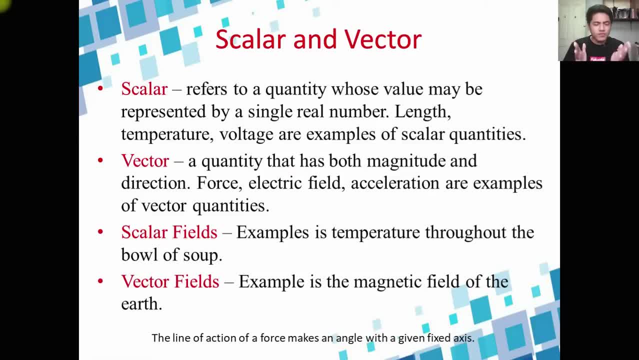 we encounter it already on our physics subject, But it is very important that we have to recall these concepts. What is scalar? A scalar is a quantity whose value may be represented by any single real number. So scalar quantities are also quantities that has only magnitude. 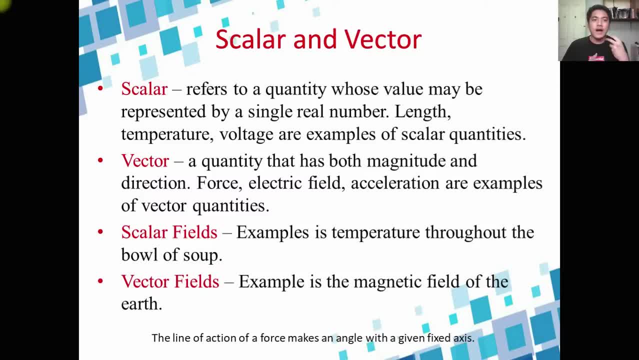 okay, Never a direction, because a quantity that has a magnitude and direction is what we call the vector, But without the direction, only the magnitude. that is what we call the scalar. So some of the examples of scalars are: length- okay, It does not have any direction. Temperature, well, of course, Voltages, These. 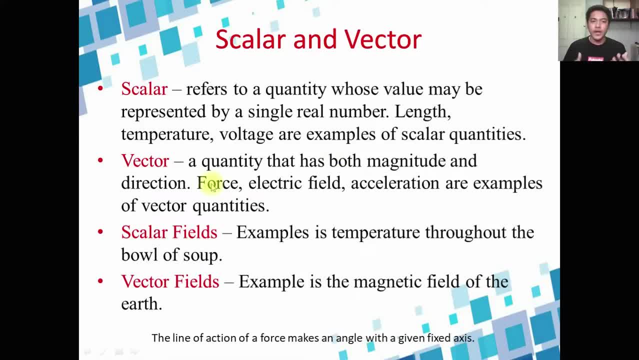 are examples of scalar quantities. Now, what for vector? So for vector, we have the force acceleration due to gravity. okay, So always going down electric field. For a positive charge it always emanates outward And for a negative charge emanates inward. So acceleration, acceleration due to. 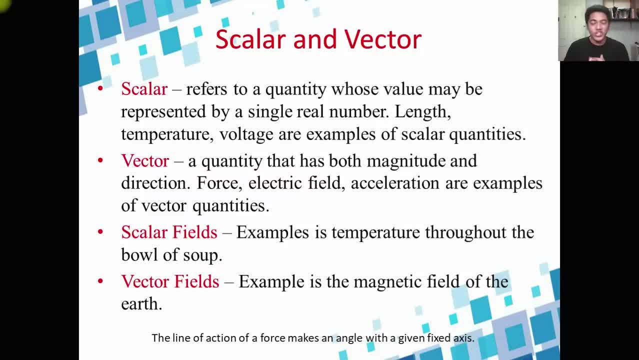 gravity- Those are examples of vector quantities- which has both the magnitude and direction, okay. So we have also what we call the scalar fields, okay, And the vector fields. well, of course, example of scalar field is a temperature throughout the bowl of soup. 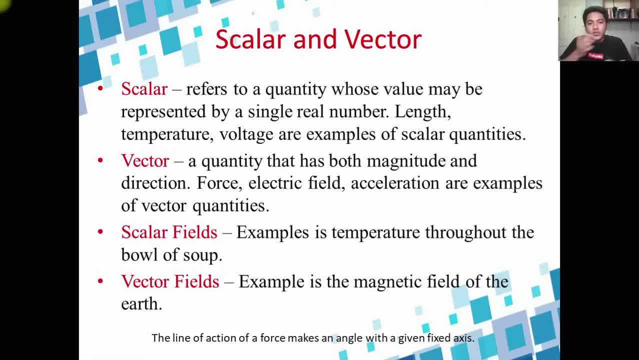 Okay, Bowl of soup. So all throughout the bowl of soup the temperature is actually constant. That is a scalar field. okay, We can actually get the direction of the temperature because it's a scalar quantity. But for, for example, for the magnetic field of the earth, 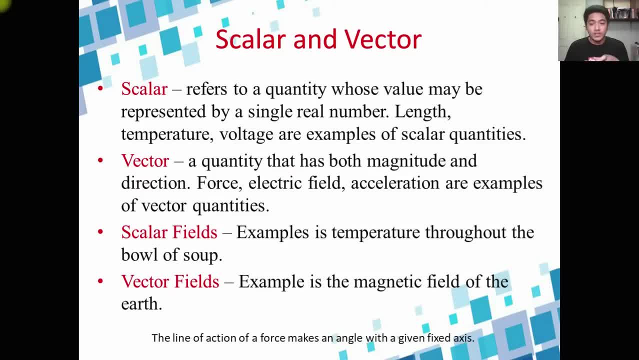 at any point. let's say, if we're going to put it into a coordinate system, there is the magnetic field of the earth. It varies from any point of the coordinate, as well as, of course, its magnitude and direction. okay, So magnetic field, so that is an example of a vector field. So vectors in our 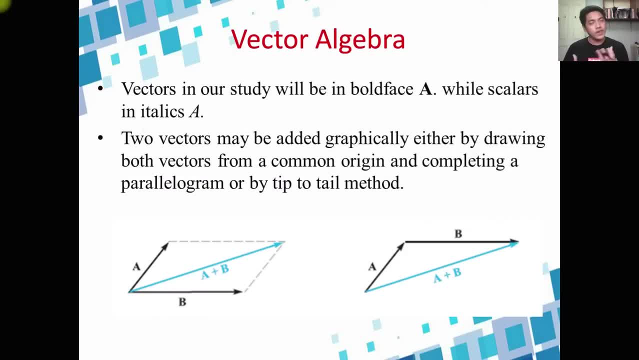 study will be always in both phase, Though sometimes vectors are actually represented by an arrowhead: okay. A letter, a quantity or a variable with an arrowhead, okay, While scalars in italics, okay. So vector algebra. so we can always add, subtract, multiply a scalar multiple. 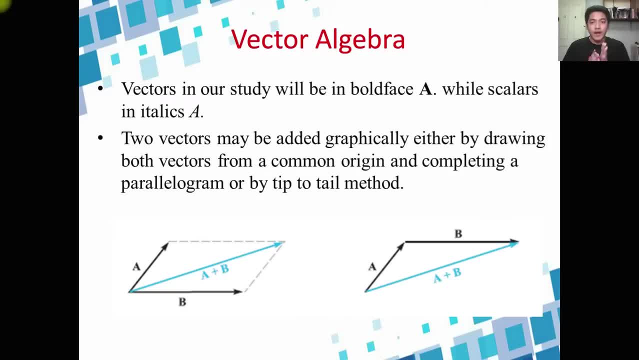 a vector. okay, So two vectors may be added graphically, either by drawing both the vectors from a common origin- which is this the common origin- and completing a parallelogram, or by tip-to-tail method. So we can add vectors by parallelogram method. This is the. 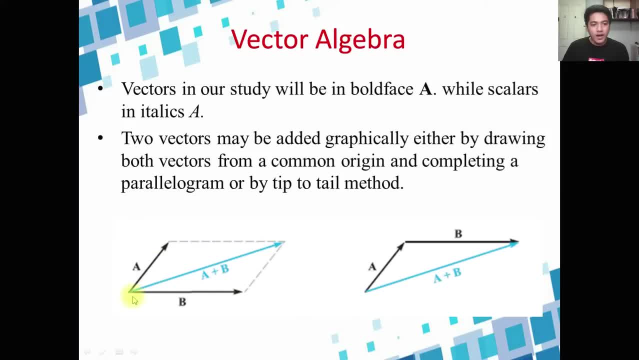 vector a, vector b. As you can see here, the resultant or a plus b, is drawn from the origin, common origin of both vectors a and b And drawn towards here, because this line, dashed line, is a projection of b and this dashed line 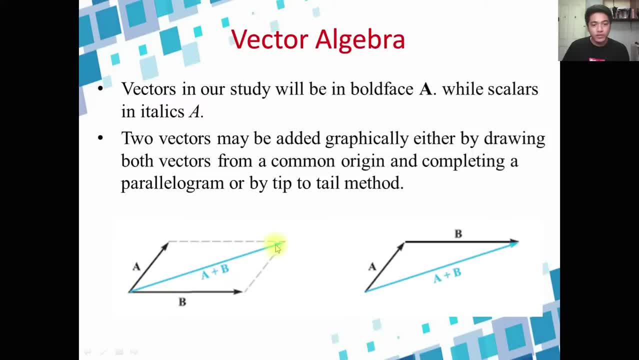 is against the projection of a, so that it's a plus b is the vector here. So hence you are forming a parallelogram, And another one is the tip-to-tail method. We can always freely move the vectors anywhere in point in space, given that we are not actually trying to change its magnitude and 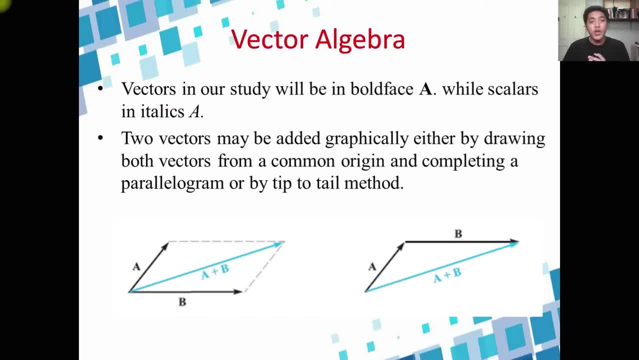 direction. As long as we are not changing the magnitude of the vector, we are not changing the direction of the vector. We can always freely move them in a coordinate system. So in this example vector is chosen as the first vector, so by tip-to-tail method. 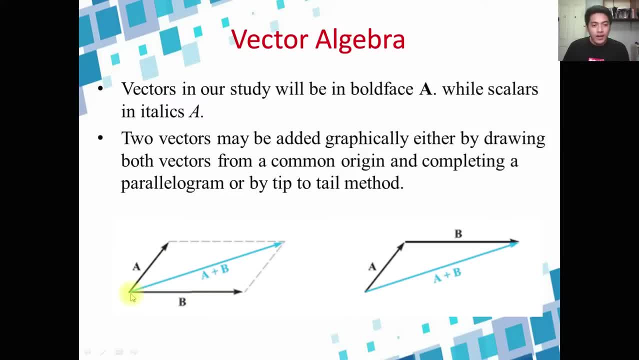 we're going to attach the tail of vector b on the tip of vector a. okay, Such that it happens. This, this image, is the result of that. So the tip of vector the, the tail of vector b, connected to the tip of vector a, and then from the very first tail, 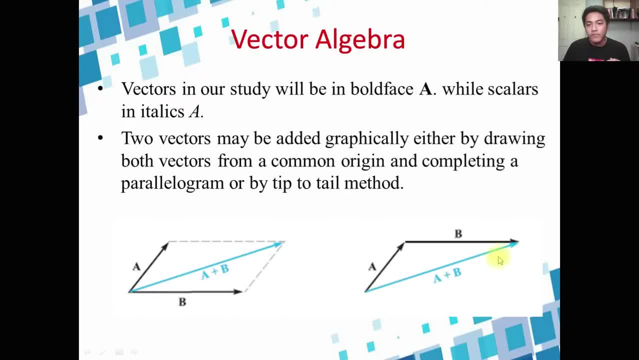 of the first vector, which is the vector a, down to the very last arrowhead, okay, or tip of the very last vector, that is, the vector a plus b. that is what we call the tip to tail method and and we can also use. we can also choose vector b as our first vector and then move this vector a. 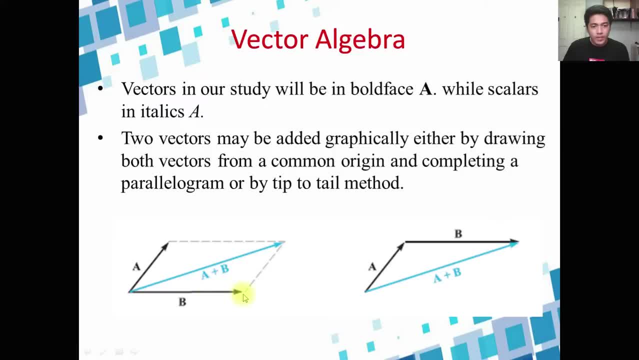 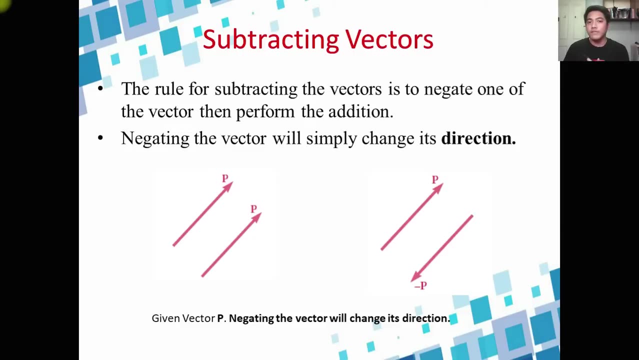 such that its tail is connected to the tip of vector b, and hence we are still having the same vector, a plus b. so in any way we can always add them from tip to tail or by parallelogram method. so the rule for subtracting vectors okay is to negate one of the vector, then perform the addition. 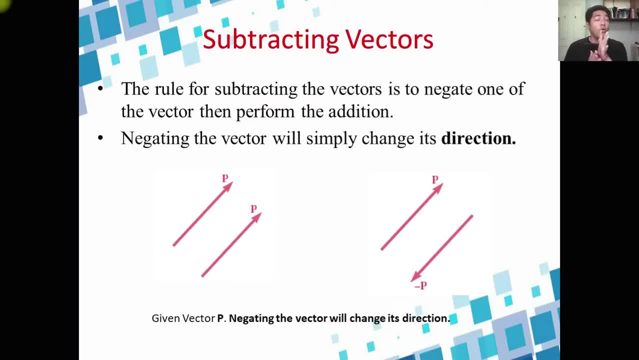 so negating the vector only means that we are always changing its direction. okay, so, such that we have an equal vector p here. if we negate one vector here such that it becomes it become negative p, it only changes its direction. okay, so it would not affect its magnitude, meaning the length of. 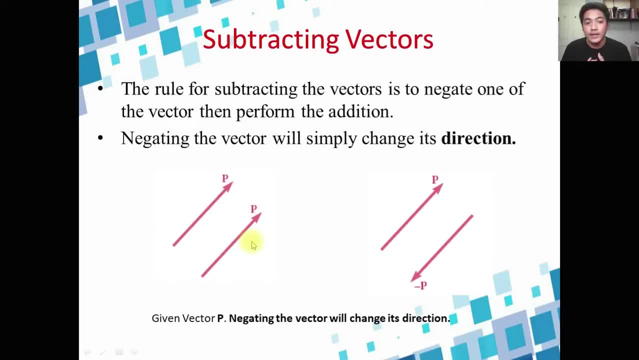 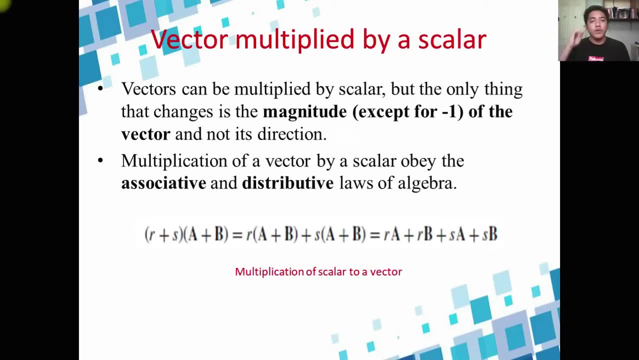 the very vector, because we only multiply negative to our vector. okay, so that's the meaning of negating the vector. it simply changes its direction. so vector can be multiplied by scalar right, but the only thing that changes is the magnitude, except for negative one, of course. if we multiply a scalar multiple of any number to a 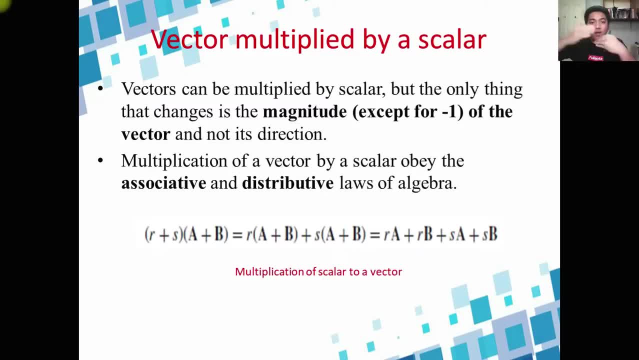 vector, it always changes the magnitude, meaning the length of the vector. okay so, and if we multiply, again negative one, well, of course it changes its direction. and as well as, if we multiply and then any negative number, it changes its direction and, of course, its magnitude. okay so, multiplication. 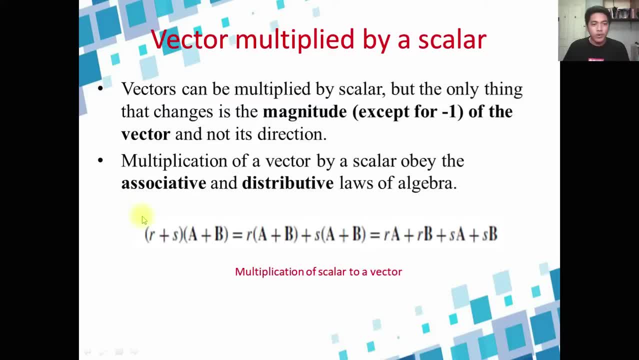 indicates that when we multiply by reading, we actually negate any vector and say, okay, so we can implement these types of measures. however, we can also spider tape. yeah, so this is what you get if you look in this class. If this is the case, 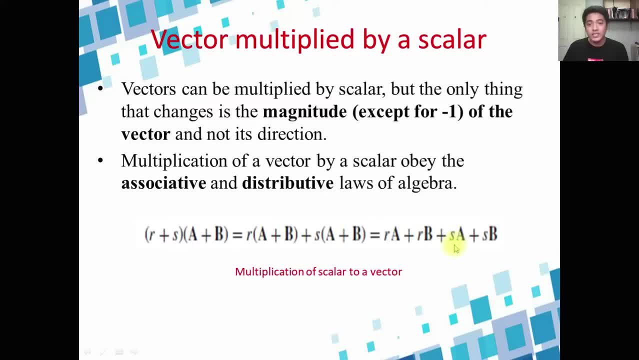 a plus r multiplied by vector b, plus a plus s multiplied by vector a plus s multiplied by vector b. note that this r and s are scalar, meaning they are actually, uh, real numbers. it can be a negative or positive numbers. the only thing that affects the, the vector, when we multiply it by a. 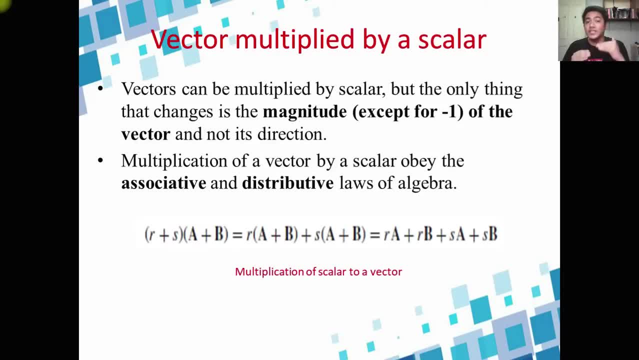 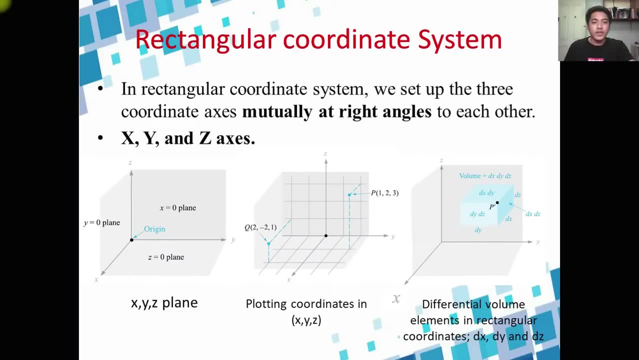 scalar one e, okay again, it only affects the magnitude, except for a negative value of scalar okay, which affects its direction. okay, so in rectangular coordinate system, in dealing with electromagnetics, we have the three uh rectangular system. so what will happen here is that we have x, y and z- okay, plane and the the relationship with 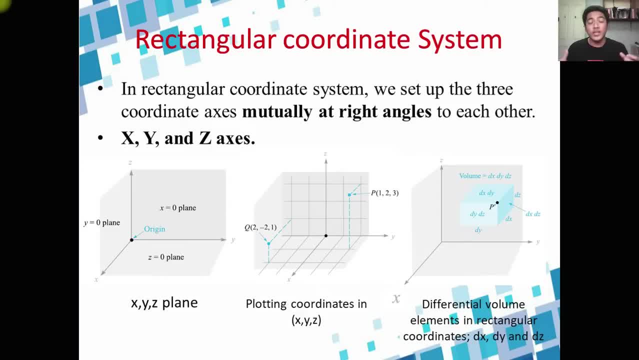 this x, y and z plane is that they are mutually at right angles to each other. so meaning, if we form, if we get the angle from x to y, that is 90 degrees. okay, if we get the angle from y to z, that's also 90 degrees. z to x, that is also 90 degrees, so that they are mutually right angles at each other. so 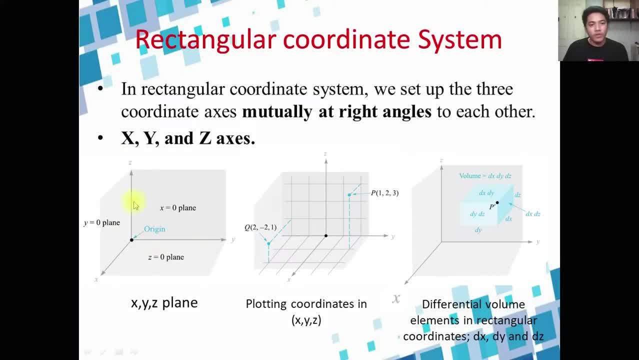 we chose here the origin as the intersection of all the points of x, y and z. so this would be: the z plane is equal to zero if we have a point lying solely in this. so if in this, lying solely on this, we have an x is equal to. 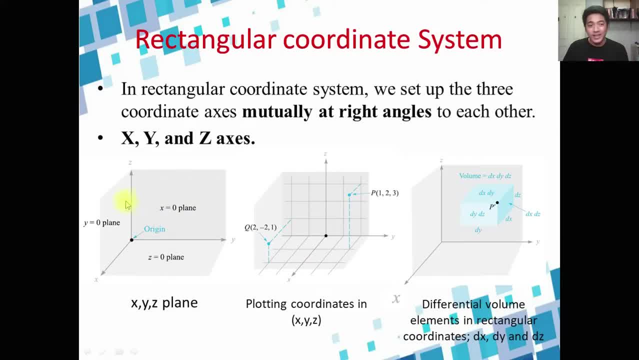 zero plane. okay, so purely on the y and z. and if we have a point here y is equal to zero plane, okay, the the, uh, the point always lie on the z and x axis only. okay, so plotting coordinates, so it is very simple to plot coordinates x, y and z. it is also always uh, also as a similarity, when we are plotting points in x, y. so for example, 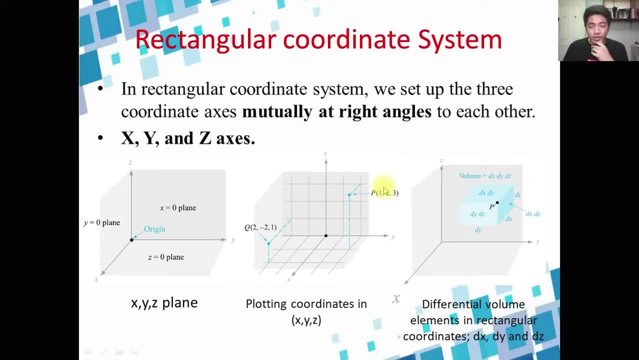 let's try to plot these points: one, two, three. so meaning one, okay, one unit, okay, positive unit- from the origin to the x. this is this, this is that okay, this is one, okay, then two units from the y. so basically, here we have one, two- this is the one, two, zero, but it has a three value of z. so you're going to step up three times. 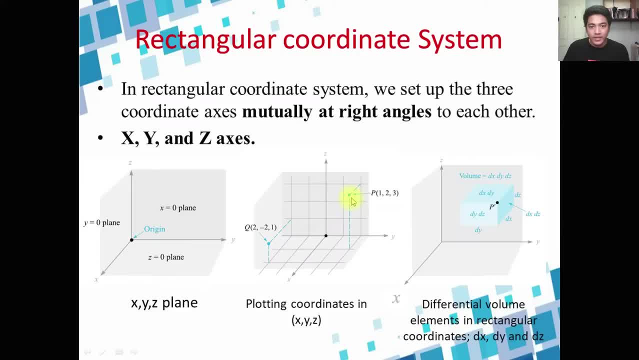 ago, because this is one, two and three. so hence this is the point: one, two, three. so that is how we plot x, y, z coordinates. okay, so, given that you have a good, uh, well, of course, sketch and, uh, dimension, a consistency in graphing these points, so of course the same for q: 2 negative 2: 1. so we have 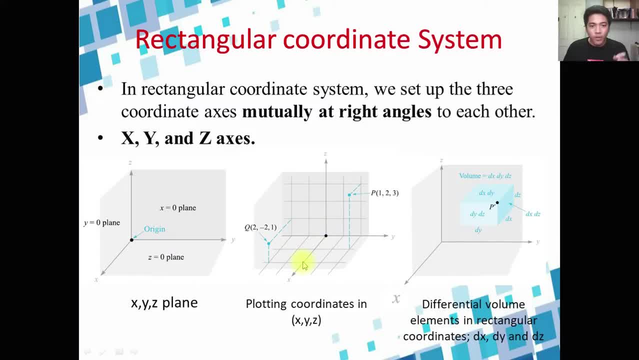 x of 2, which is this negative, 2 of y, so 1, 2 to the left of the y plane is the negative. then, of course, one step ahead of z, okay, so here is the point: negative or 2, negative 2 and 1, and of course we. 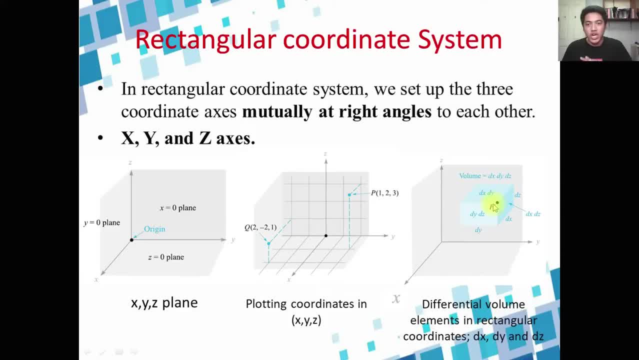 have also the differential volume. if we take, for example, a differential uh values of dx, dy and dj, we will be arriving at the differential volume of this, wherein our volume is simply uh, we will get dx, dy, dj. we multiply that so it it actually corresponds to a uh, let's say a cube. okay. 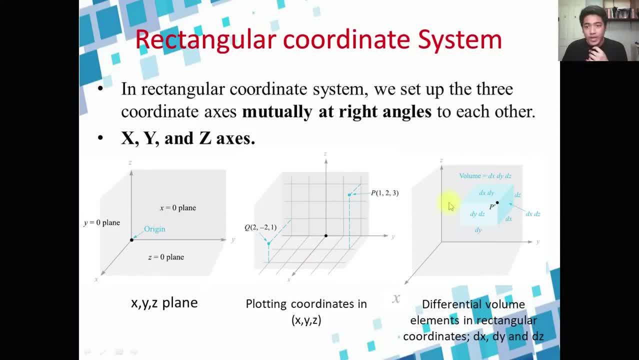 because the volume is dx, dy, dj. so if we make a cube using dx, dy and dj, as we can see, we have a point here. and if we make a cube using dx, dy and dj, as we can see, we have a point here. so this point will become dy, dj. why? because it's it only shows the y and z. okay, if, if that point is. 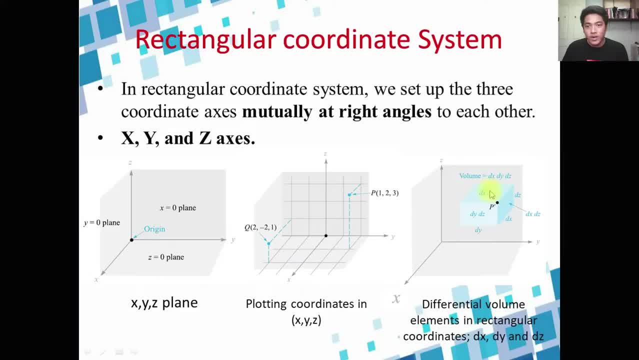 in, in the side of the space of the cube. dx dy here. because why no z? because there is no height in here and we have here dx dz. why? because there is no y direction in this phase of the cube and, of course, the the horizontal is d. 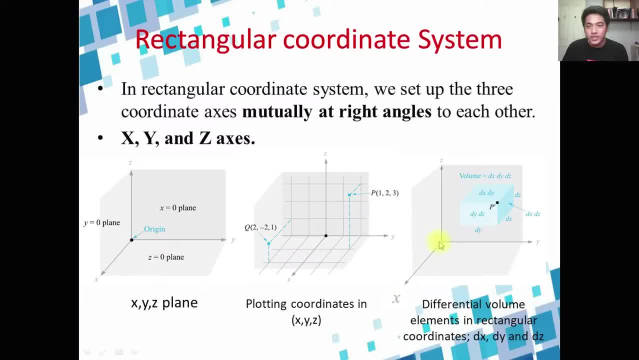 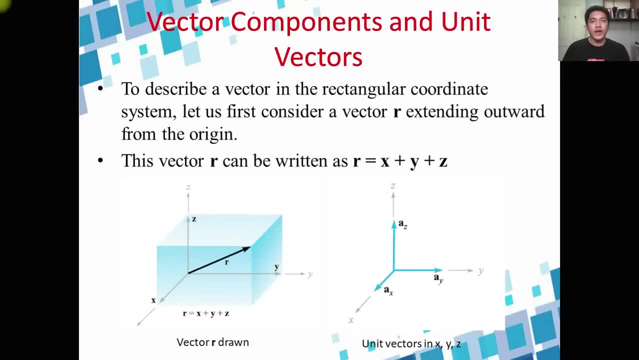 y. this line is dx because it corresponds to this, and dj is the height, which corresponds to z axis. okay, so vector components and unit vectors. so to describe a vector in the rectangular coordinate system, let us first consider a vector: r, so vector, are extending toward from the origin. so this vector are extending to, from the origin, toward any point in the x, y, z plane. 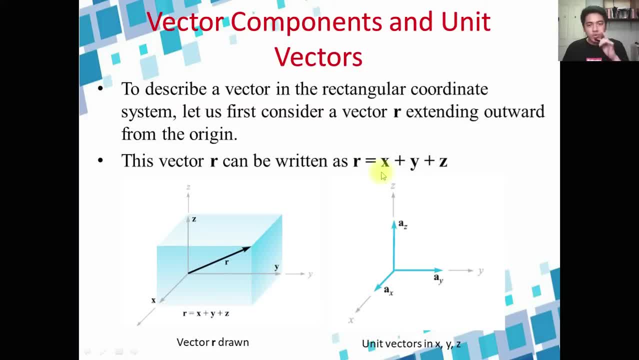 can be rewritten as vector r is equals to x plus y plus z, so vector r drone. why? because if we get again by vector analysis or by vector addition of vectors, okay, we have x here. if we move this vector x here because we have x here, we move this vector x here such that we place the plane of this vector. 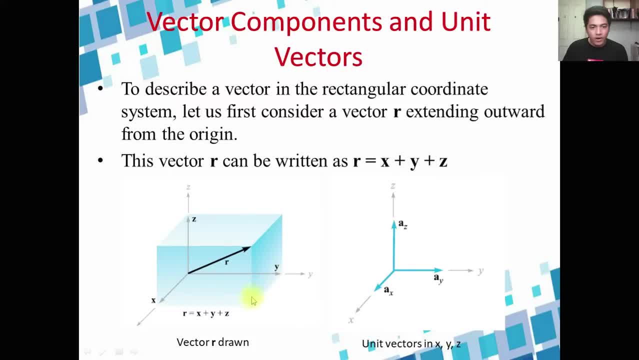 x to the tip of vector y. here is our vector, but take note, you also have z here, so that if i'm going to move this z here and place its tail to the tip of vector x here, connected here, i will be having this vector, okay, such that i form a triangle, and by the vector. okay, by. 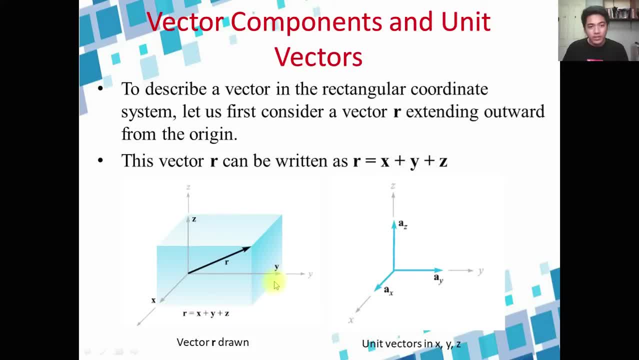 the vector addition using tip to tail method. we're going to draw the vector r from the very tail of the first vector, which is y, up to the the tip of the very last vector, which is z. so, as you can see, that is the vector drawn: x, y, x plus y plus a. okay, so we have also unit vectors. 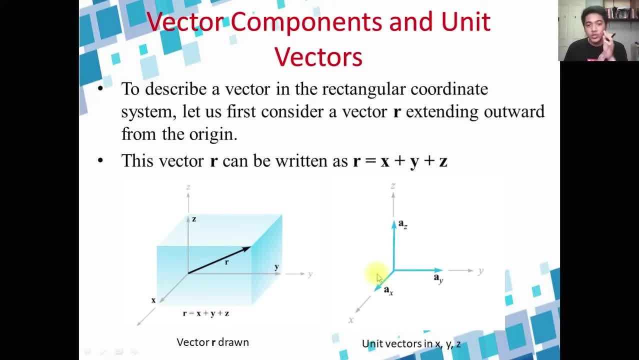 unit vectors are actually the vectors that has a magnitude of one, okay, hence the term unit. so in this study, uh, we're going to have vector you, vector unit vectors in x, y, z as a x, a, y, a, z to denote that that is a unit vector. okay, finding the vector from two points. 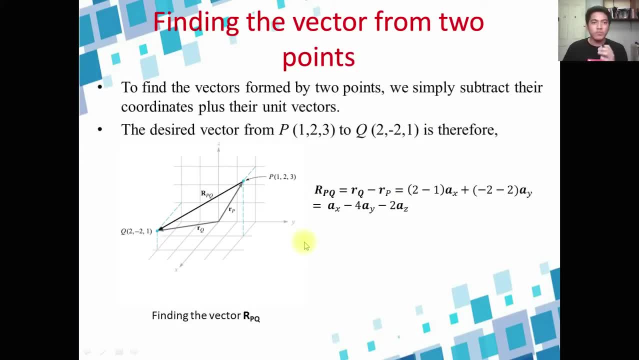 so to find the vector formed by two points, we simply subtract their coordinates plus their unit vectors. so for example, we want to find: we are given two points in the x, y, z plane coordinate, so we have one, two, three, two negative two, one. so if we're going to get the vector from point p, 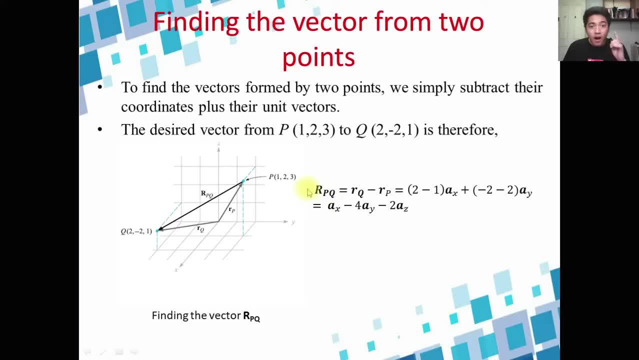 to point q, hence denoted by r, r sub p, q. so it means from point p to point q. what are we going to do is to simply what subtract their unit vectors. our unit vectors is, from the origin, r sub q and r sub p. well, of course, how do we get that? r sub 1 and r r sub q and r sub p. 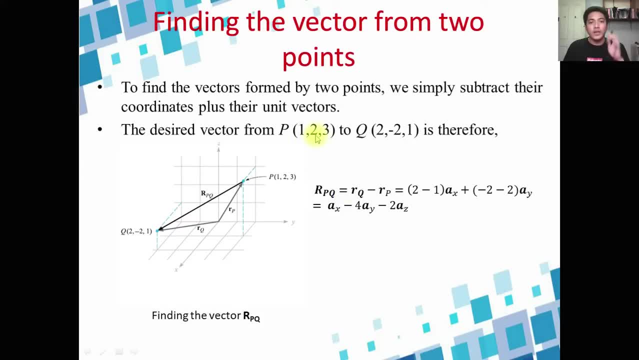 but of course from the origin. so, one minus zero, two minus zero, three minus zero. okay, hence, that is the r sub q, r sub q, okay, and r sub p is this? so what are we going to do is simply to get the vector emanating from r or from p to q. we simply what subtract, its uh coordinate, and we're going to 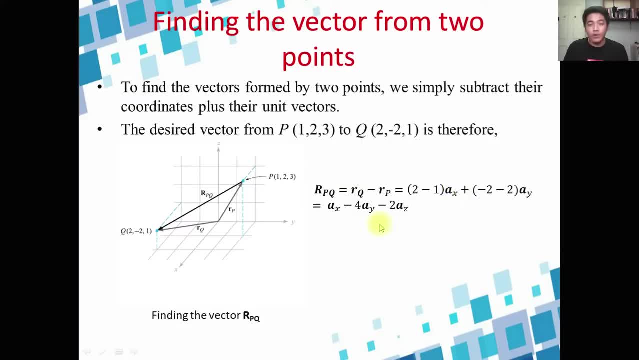 put vector of unit vectors a, x, a, y and z. so in this case, if we want to get the vector from p to q, we're going to subtract 2 from p to q. So it means the terminal point is the cube. So that is the first one we're going to subtract. 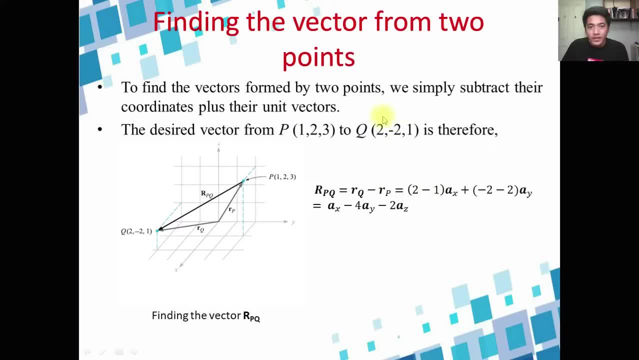 So we have 2 minus 1.. We have negative 2 minus 2.. Okay, that is plus. Okay then 1 minus 3.. Okay, I forgot to write the 1 minus 3 here. So what will happen here is 1 minus 3 az. 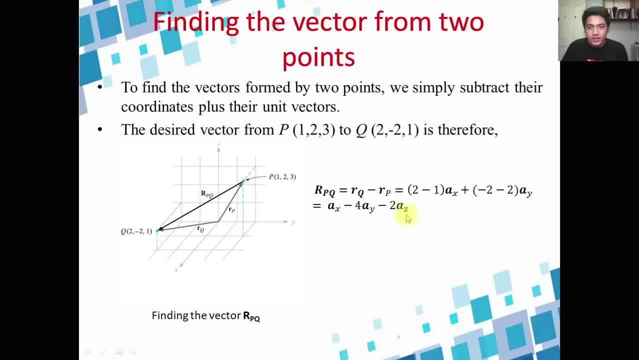 So we have a sub x, X negative. 2 minus 2 is negative 4 ay. Okay then 1 minus 3 is negative, 2, az. Hence the vector from r or from p, from point p to q, is given by this vector. 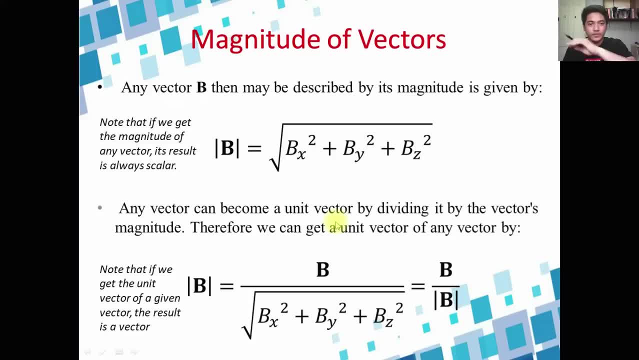 Okay, so that's how we find the vectors. So we have what we call the magnitude of the vectors And the unit vectors. okay, So any vector b then may be described by its magnitude, given by this equation. So magnitude is represented by, like an absolute value. 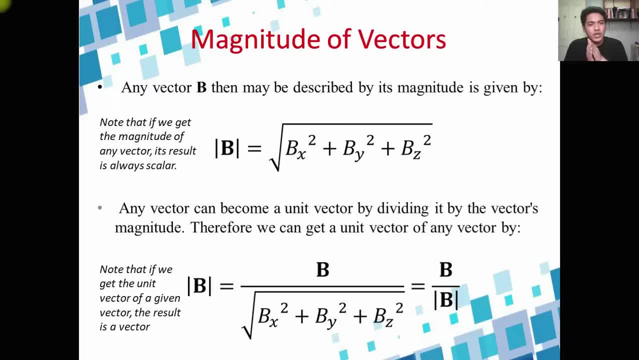 Okay, but me, when I'm teaching vector analysis, I always use the double absolute value, let's say, to denote that it is different from the absolute value. Well, by the book. it says that if we have an absolute value, let's say a parallel line in between or inside. 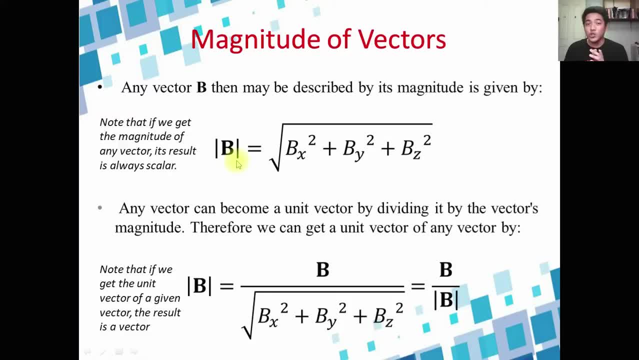 and inside of that is a vector. so that denotes the magnitude of vectors. So what is the magnitude of vector? Again, if we're going to go back, the magnitude of the vector is the length of the vector. So we can get the magnitude of the vector by this formula. 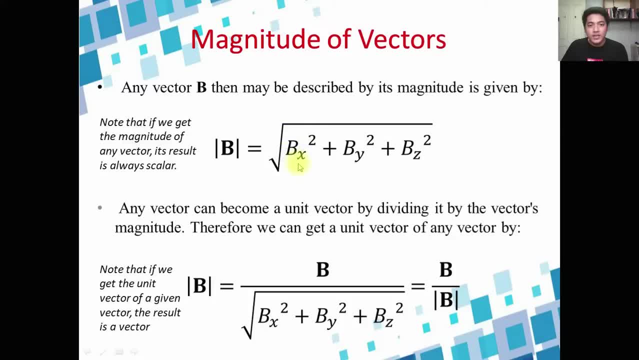 We have the square root of the x squared component, scalar component of the x, plus the scalar component of y squared, plus scalar component of z squared, and then we have the square root. Note that if we get the magnitude of any vector- okay, if you're going to get the magnitude of any vector- 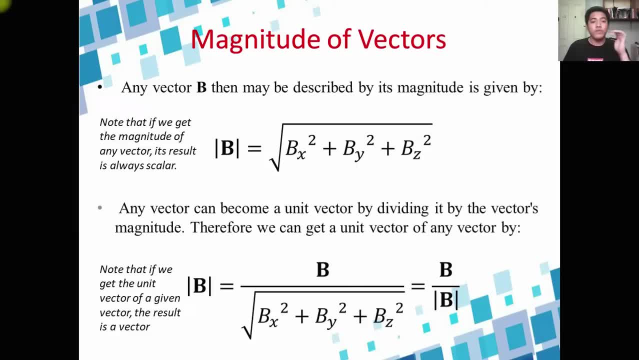 the result is always a scalar quantity. okay, So we have now what we call the unit vector. again, How do we find a unit vector? okay, from a vector. okay, So any vector can become a unit vector by dividing it by the vector's magnitude. 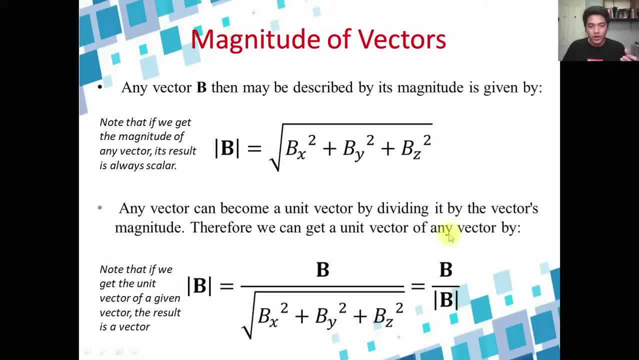 So therefore, we can get a unit vector of any vector. okay, If we want to get a unit vector of any vector, we can use this formula. okay, We can use this formula. meaning is that? no, it's actually. this is not magnitude of b, okay. 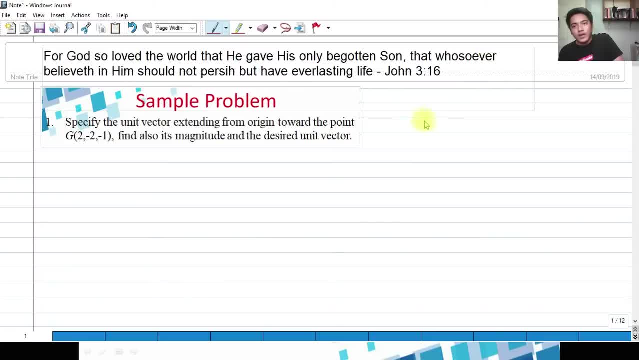 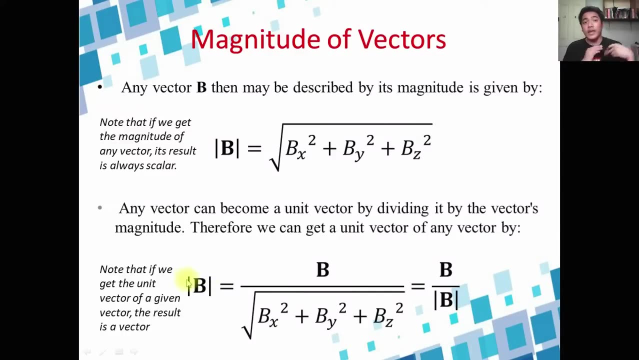 This should be written as: okay. this should be written as a b. okay, That denotes the unit vector. okay, Pardon me. Okay, this should be rewritten as a sub b to denote a. that is a unit vector. okay. 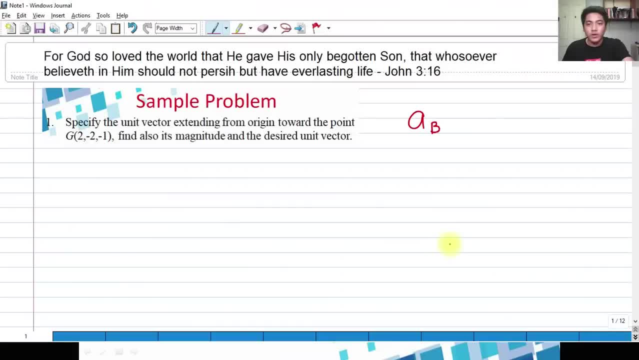 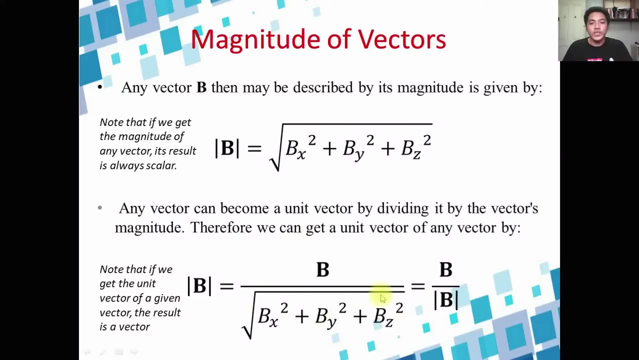 So in order for us to get the unit vector of any vector- a sub b denotes the unit vector- we need to have the vector divided by its magnitude vector. okay. So, as you can see here, b over the magnitude of b, okay, which is this magnitude is equal to this. 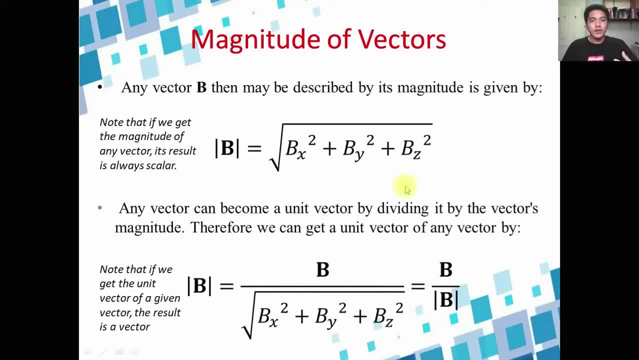 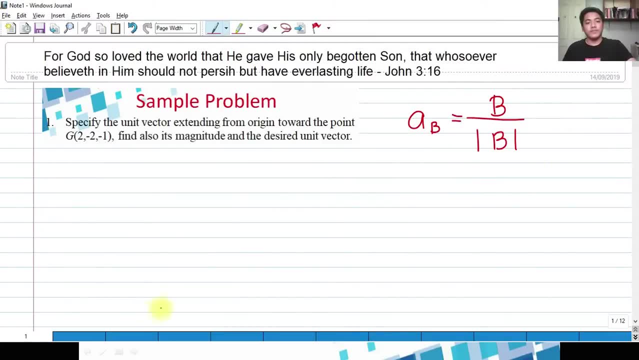 Okay, as we have shown it a while ago And again, if we get the unit vector of any vector, the result is always a vector. okay, Remember that. Okay, So let's try to have a sample problem. So let's try to solve some problems. 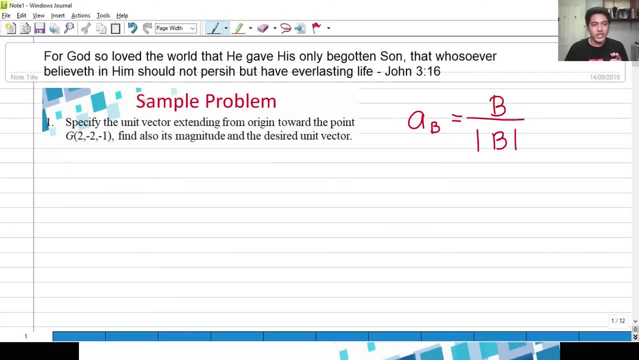 Specify the unit vector extending from origin toward the point g to negative 2, negative 1.. Find also its magnitude in the desired unit vector. So it says: from the origin, Which is the coordinates of the origin, 0,, 0,, 0, 2, point g, which is actually 2, negative 2, and negative 1.. 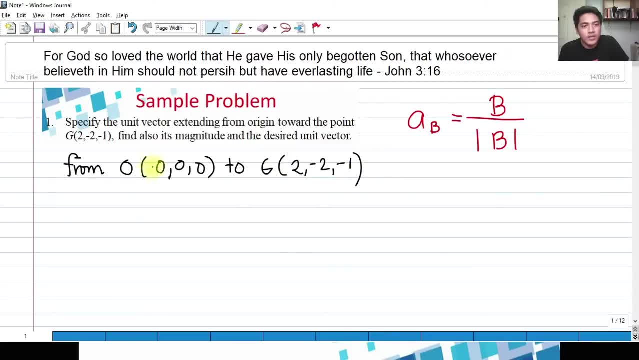 So this is our terminal point. This is our initial point. Therefore, the vector g- okay, I'll try to write this in boldface. okay, Vector g is actually. what Terminal point is this? 2 minus 0.. 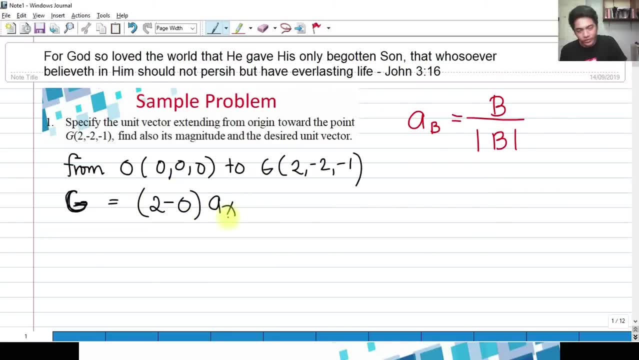 Terminal minus initial, multiplied by the unit vector ax Plus, we have terminal for y negative 2 minus 0.. We have ay unit vector Plus. lastly, we have negative 1 minus 0. az Simplifying, we have 2ax minus 2ay minus, simply az. 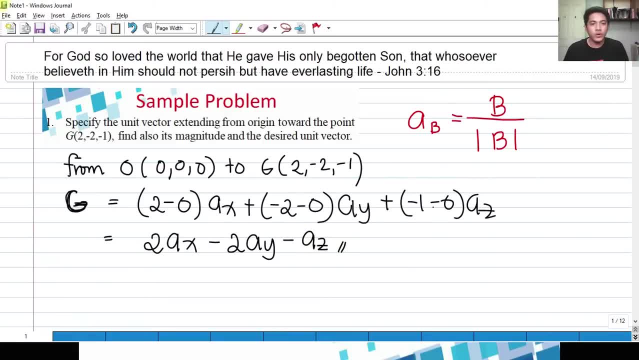 And this is the unit or the vector. Unit vector from origin toward that point g. okay, So find also the magnitude in the desired unit vector. So to get the magnitude of the unit vector we simply denote it as like the absolute value. 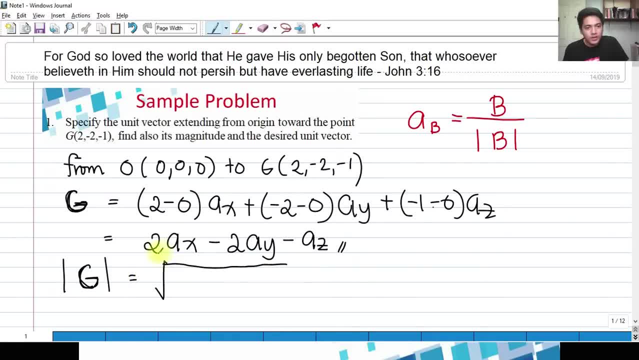 And we have the formula while ago. okay, The components. okay, We're going to add the square of the components and take the square root of them. So we have here 2 squared because of this, Plus negative 2 squared. okay. 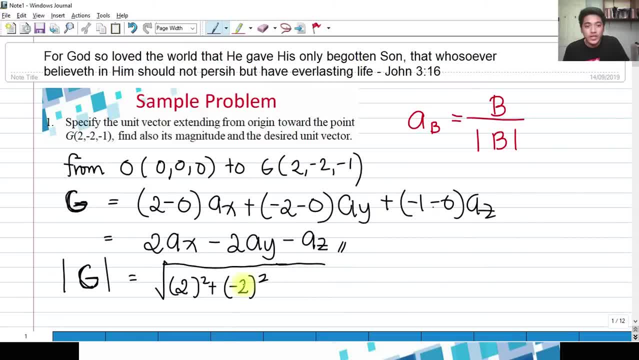 No problem, Even if it's negative, because it's raised to square. So any number raised to square, even if it's a negative, will still yield to a positive value. So plus negative 1 squared, because the component of this is negative 1.. 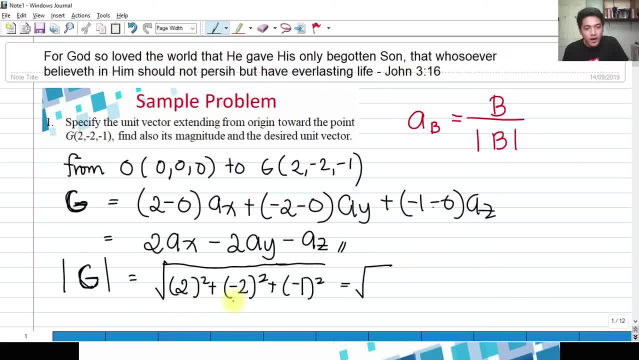 That is square root of 2 plus 4 plus 4, 8 plus 1.. That's square root of 9.. And that's equivalent to 3.. That is the magnitude of the vector. That is the magnitude of the vector g. 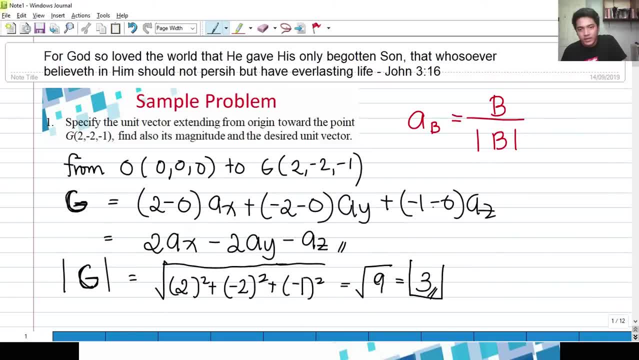 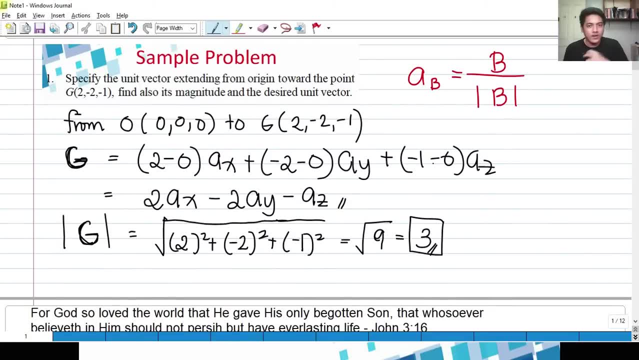 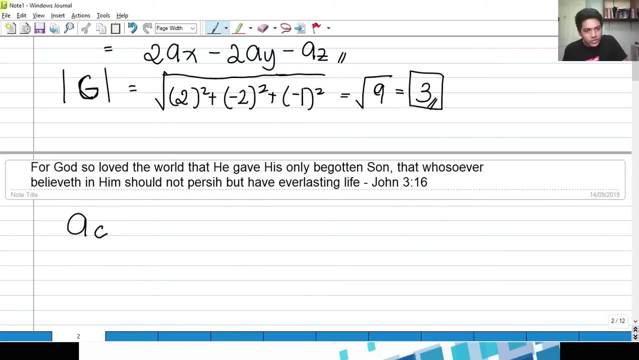 As you can see, this is a scalar quantity. okay, This is a scalar quantity because if we take always the magnitude of any vector, it's always a scalar quantity. How about the desired unit vector? The desired unit vector, okay, of a to g. okay, is actually equal to what? 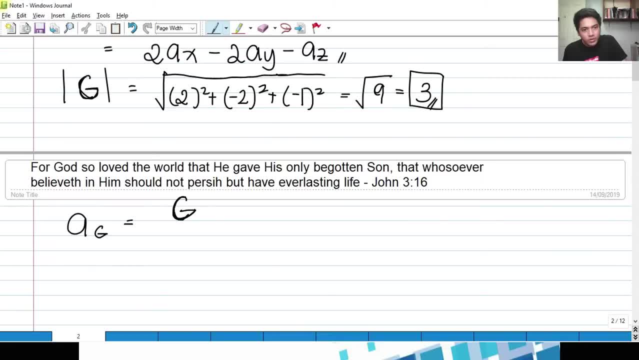 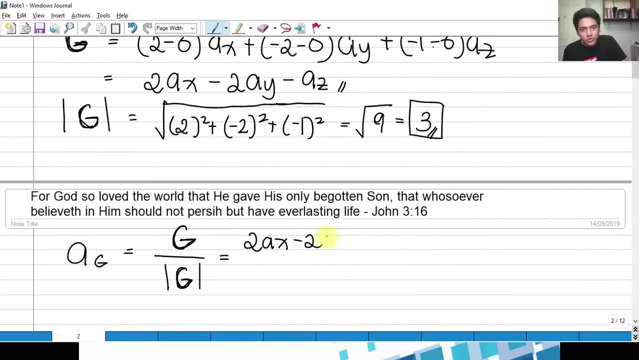 The vector g itself. okay, The vector g itself. over what? The absolute or the magnitude of the vector g? okay. So the vector g is what This vector We have, 2ax minus 2ay minus az over. the magnitude of the vector g is 3, okay. 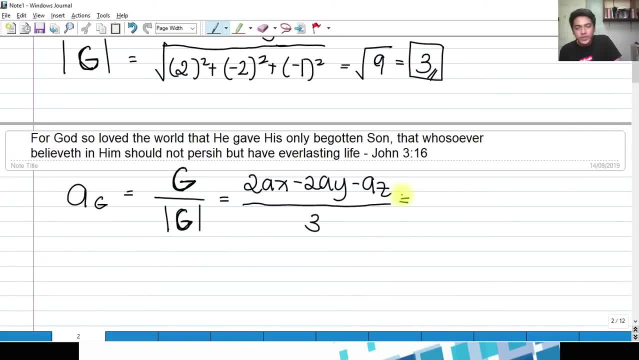 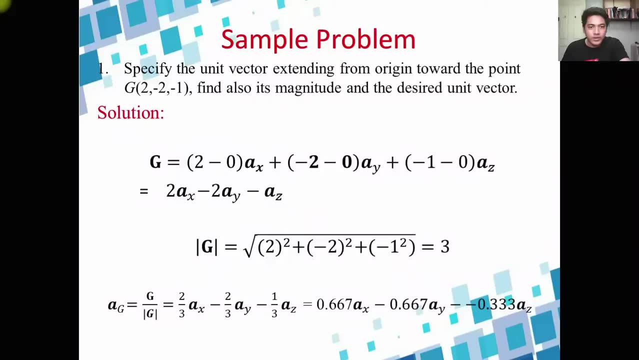 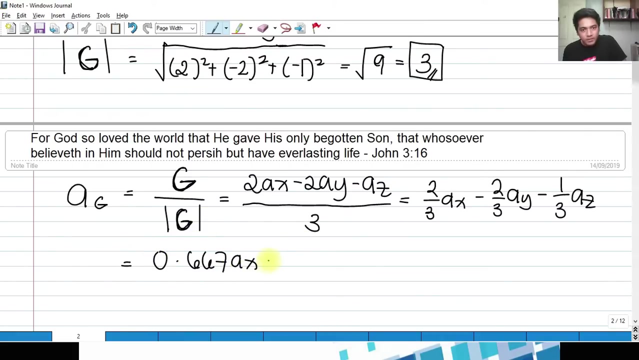 Hence our answer should be: okay, 2 thirds ax minus 2 thirds az, Or in decimal. in decimal, that is equivalent to 0.667ax minus 0.667ay, if I'm not mistaken. okay, Okay, minus 0.333az, okay. 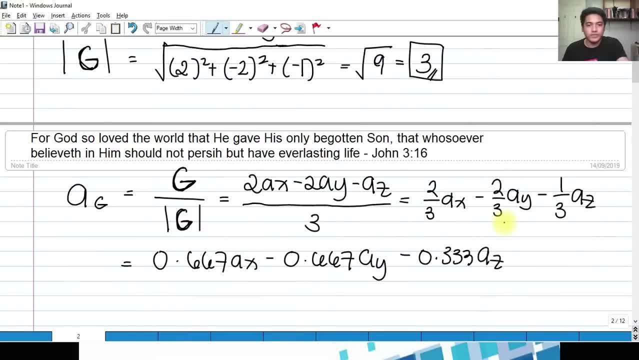 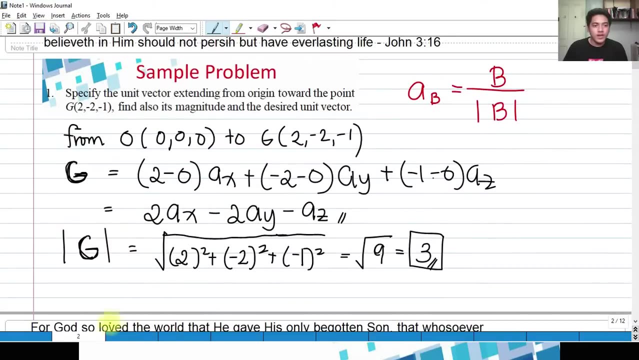 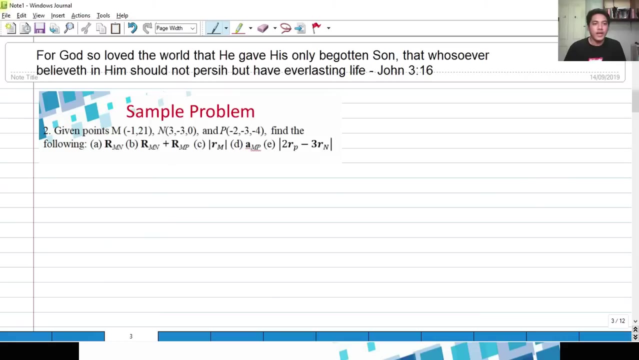 That is our answer. Okay, So this is the vector or the unit vector of that vector g, okay, Okay, so let's try again. Number 2.. We have 3 points Given, points m- negative 1, 2, 1 and 3, negative 3, 0 and p- negative 2, negative 3, negative 4.. 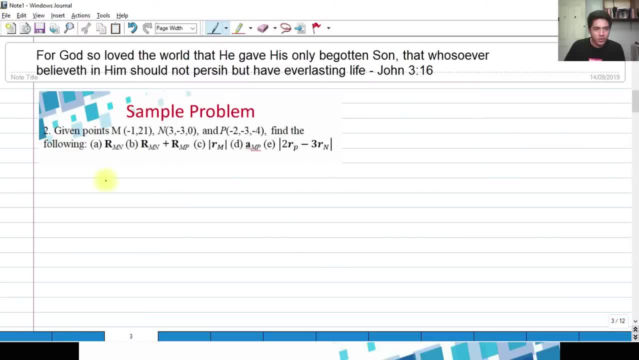 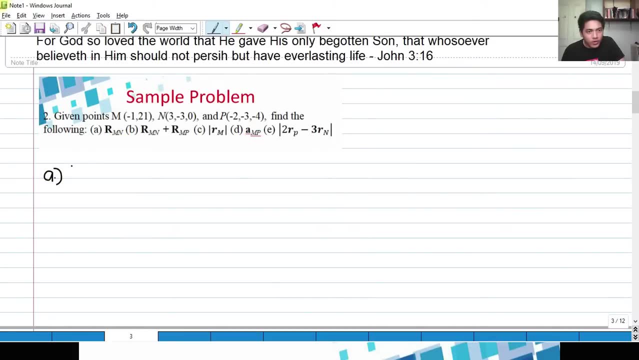 Find the following: okay, So r sub mn. So what does this mean? Okay, the unit or the vector. from m to n. okay, From n to n. So, as we can see here, from n to n. so our terminal is n. 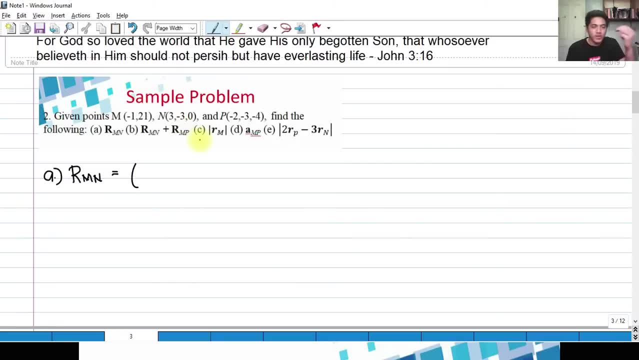 So what are we going to do is to simply subtract its coordinates and write a, what A unit vector, ax, ay and az. So what will happen? From n to n? this is our terminal point. So that means 3 minus the x component, minus negative 1ax. okay, 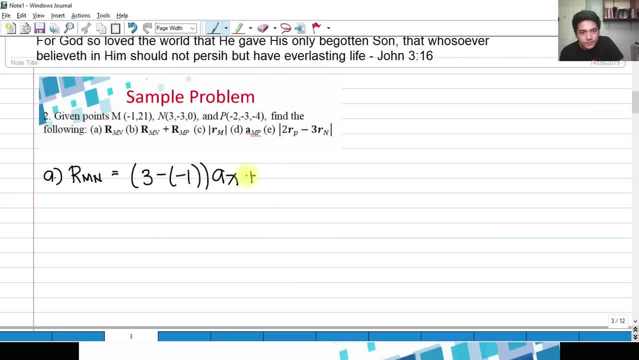 3 minus negative 1. Be careful for that. Plus, of course we have what Negative? 3 minus 2ay okay. Plus we have 0 minus 1. az, So our answer should be: negative times. negative is plus 1.. 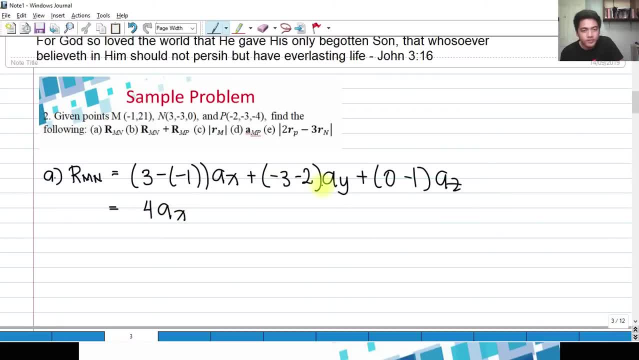 So we will be adding 4ax here: Negative 3 minus 2 is negative. 5ay here. 0 minus 1 is negative. az here. So that is the vector from m to n, okay. Resulting unit vector. okay. 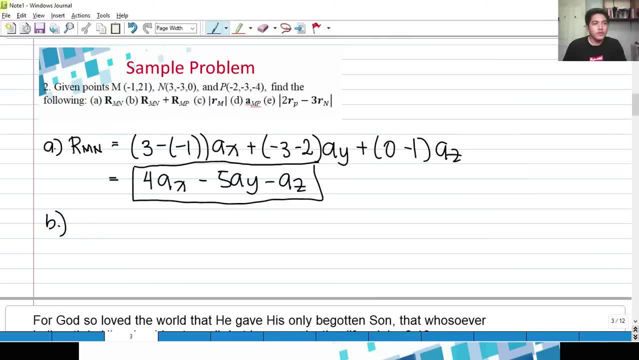 Vector from n to n. So let's try to solve the letter b. We have vector from rmn plus r from mp, r, sub mp, which means vector from m to p. So we already got the vector rmn. How about the vector rmp? okay, 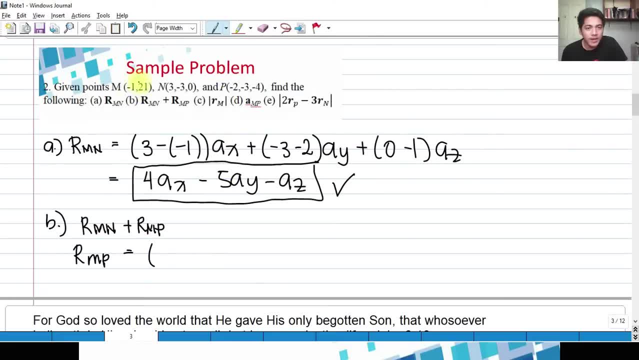 So our final point here is the p Initial is m, So we have negative 2 minus negative 1ax plus. we have negative 3 minus 2ay plus negative 4 minus 1, negative 4 minus 1az. 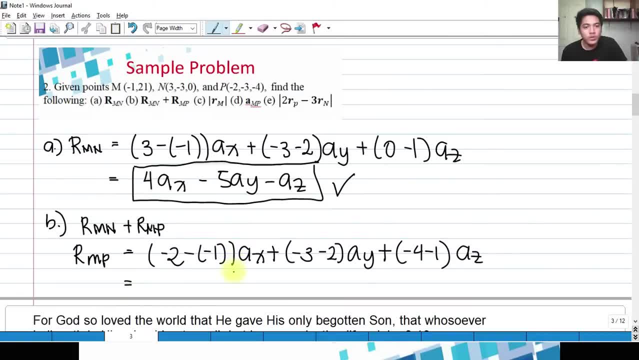 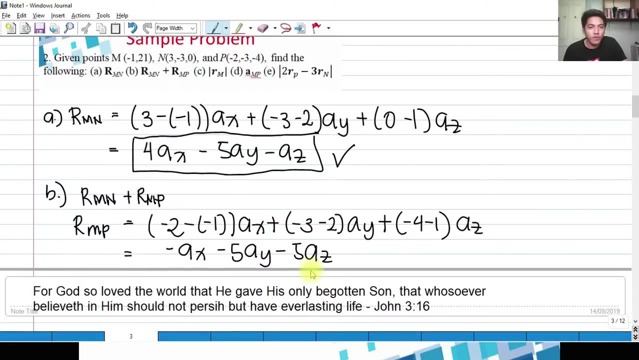 So, evaluating negative 2 plus 1 is negative ax. okay. Negative 3 minus 2 is negative 5ay. Negative 4 minus 1 is negative 5ay. So we can now perform vector rmn plus rmp by simply adding: okay. 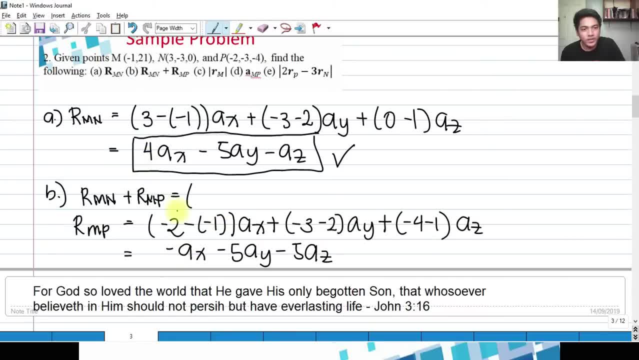 By simply adding the components. okay, So we have 4ax plus negative. ax is simply what? So that is 3ax. Okay, That is 3ax, So I will show you how. again, So the components 4 and y: 1.. 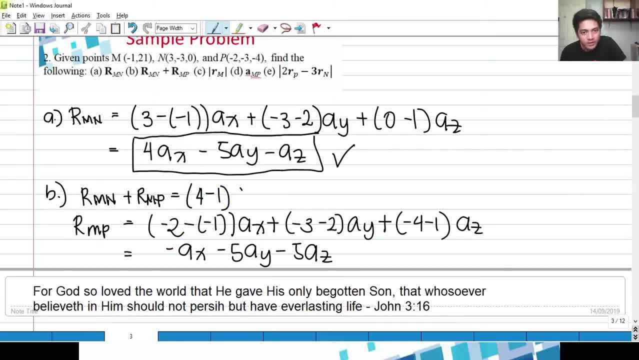 So we have 4 minus 1ax, plus we have negative 5 minus 5ay sub y, plus we have negative 1 minus 5ay sub c. Hence our answer would be 3ax okay Minus 10ay minus 6a sub z. 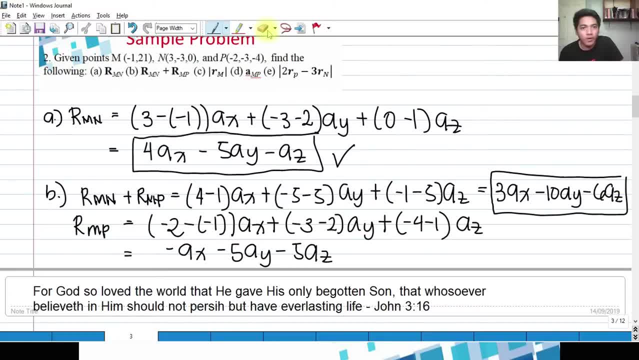 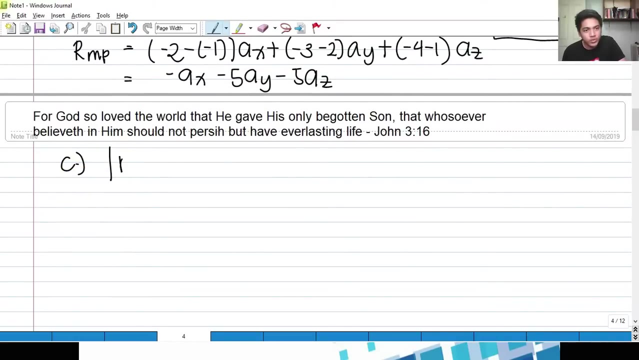 So this should be our answer for our problem, letter b. So let me just rewrite this: a sub x. okay, So a sub x. That must be our answer For letter c. it says the magnitude of the unit vector rm. 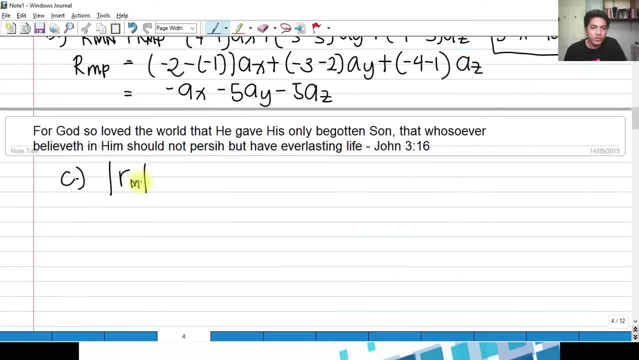 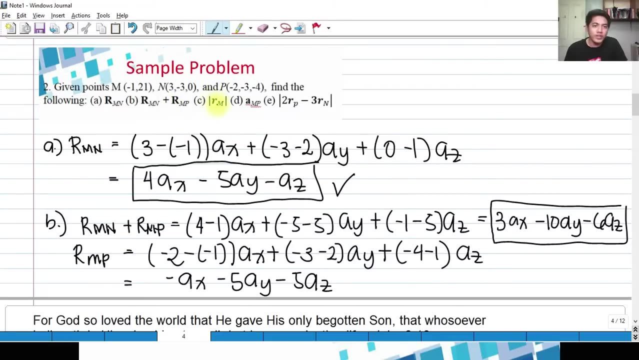 So if we see this sign, okay, It denotes that the magnitude of rm, So our result here should be scalar. But first we need to find the vector rm. What is the vector rm? It only says that your initial point here is the origin. okay, 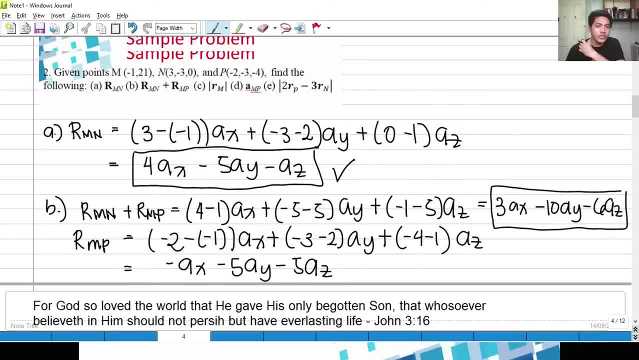 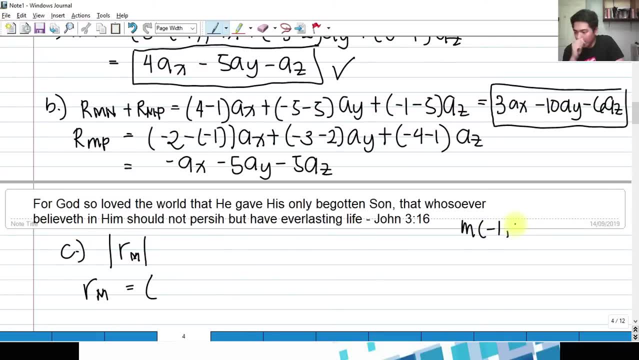 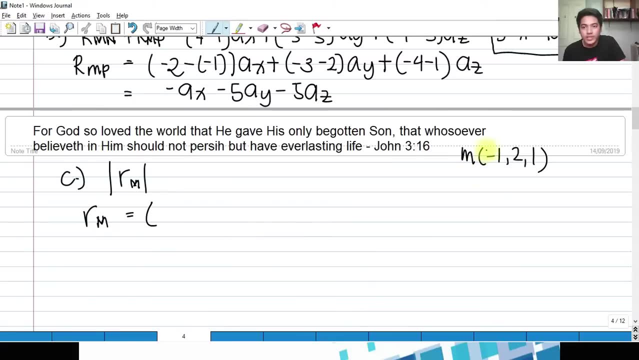 So if the initial point is the origin, your final point is m. So let's label this our m. Let's just copy negative 1.. We have 2 and 1.. So if your initial point is the origin, the final point is m. 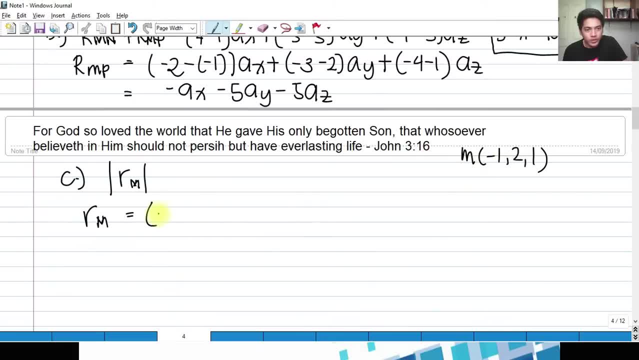 You're going to what? To get the vector multiply or minus. again negative 1 minus 0.. This is the final point. initial point: ax Plus Okay, final point of 2 minus 0, a sub y. 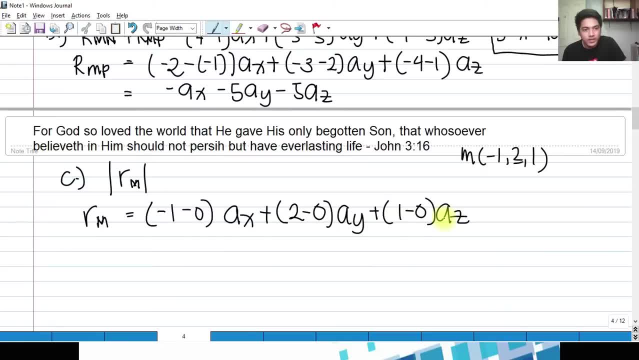 Plus final point of 1 minus 0, a sub z. So we have now negative ax plus 2a sub y- Okay- Plus a sub z- Okay, Okay. So the magnitude: We are asked for the magnitude. 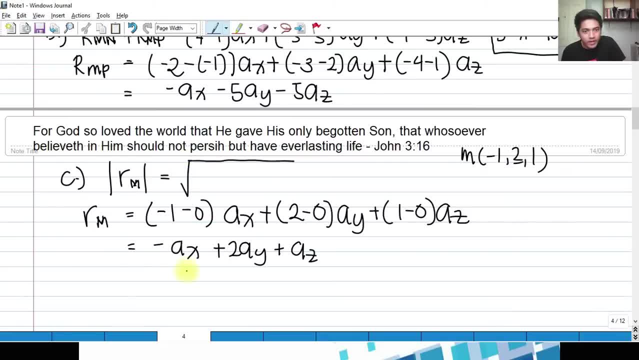 So we can get the magnitude. We have now the vector here. So what is the magnitude? Negative, 1 squared, because the value of here, the coefficient here, is negative. 1 plus 2 squared plus 1 squared And that is equivalent to, if you calculate it, 2.45.. 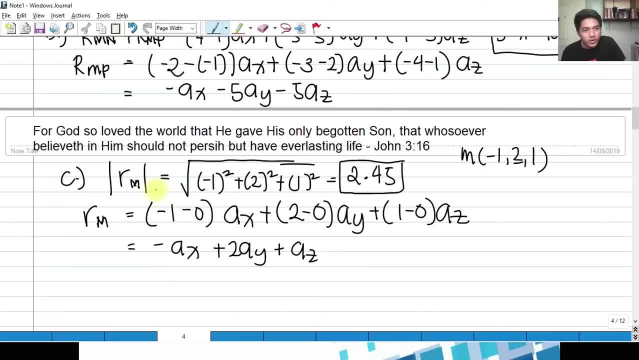 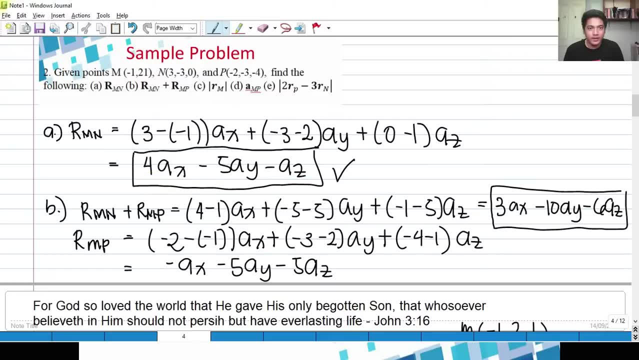 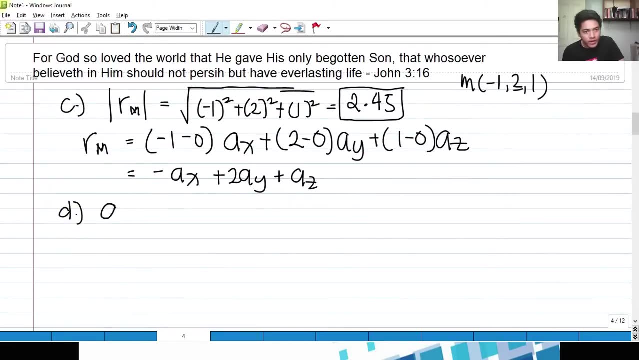 Hence the magnitude of this vector is 2.45.. Okay, And for letter d. Okay, For letter d. So we have a vector unit. vector of a m p. Okay, Do we already have m p here? 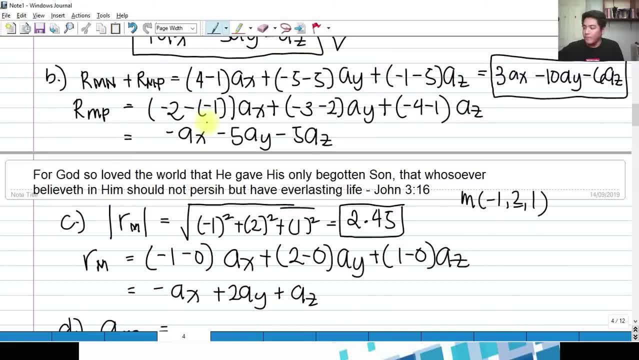 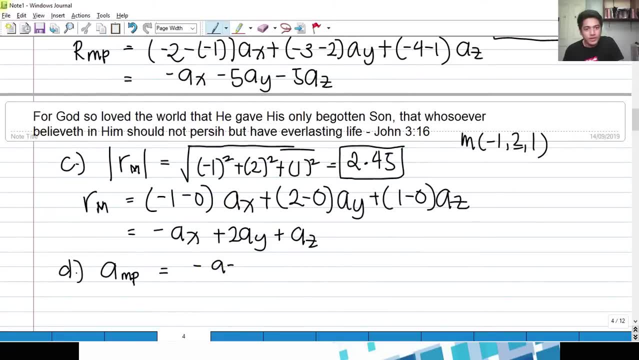 Yes, we have already the m p here And our m p vector, m p is actually this one negative ax. So we have negative a sub x minus 5ay minus 5az over. this is a unit vector. 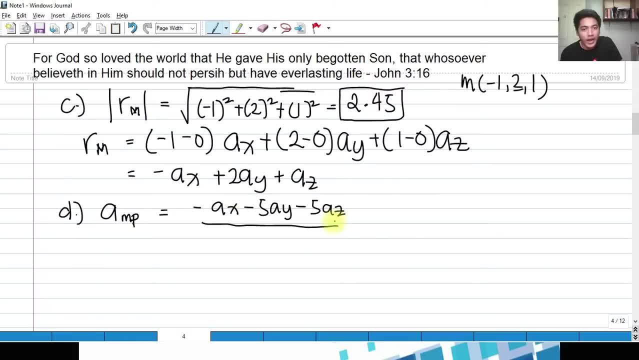 Okay, This is our unit vector. So this is the vector m, p, And remember, we're going to get the unit vector by what We have: the numerator, the vector itself divided by the magnitude of the vector itself. So what are we going to do? 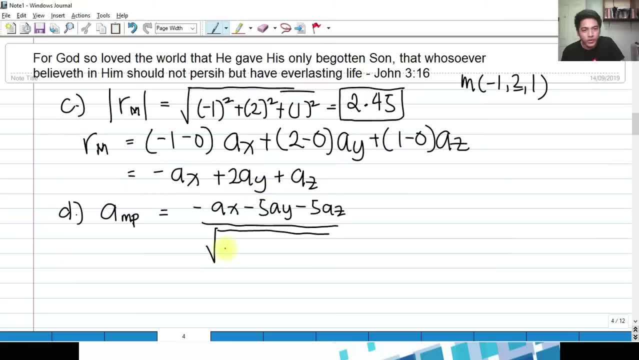 Okay, Divide it by the magnitude of this. So we have negative 1 squared plus negative 5 squared plus negative 5 squared. Okay, So if we divide that, what will happen By your calculator? okay, 5az, this should be square root of 51.. 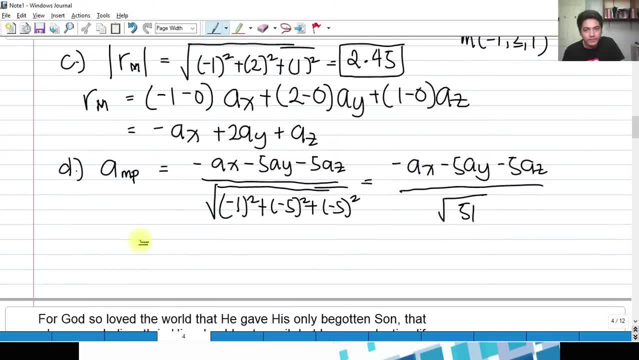 Okay. So if you calculate that we have negative 1 over square root of 51ax minus 5 over square root of 51ay sub y minus 5 over square root of 51ay sub z. Okay, So if you simplify this, your calculator would give you what. 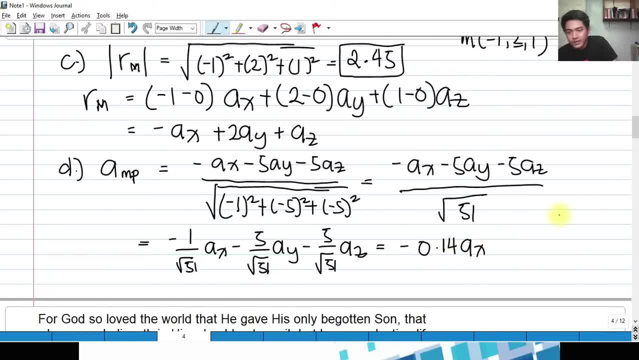 Negative 0.14 a sub x. negative 0.7 a sub y, minus negative 0.7 a sub z, And this is the desired unit vector of m p. Okay, The vector m p. I hope you can follow what I'm trying to say here. 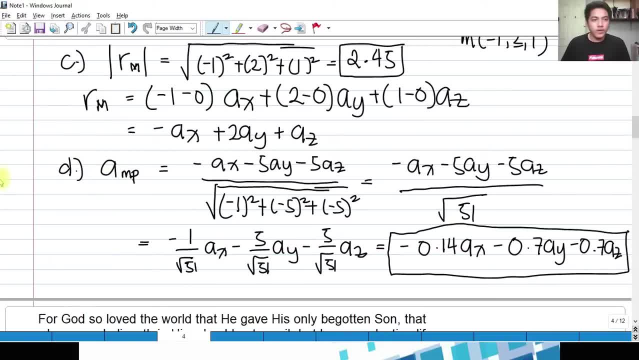 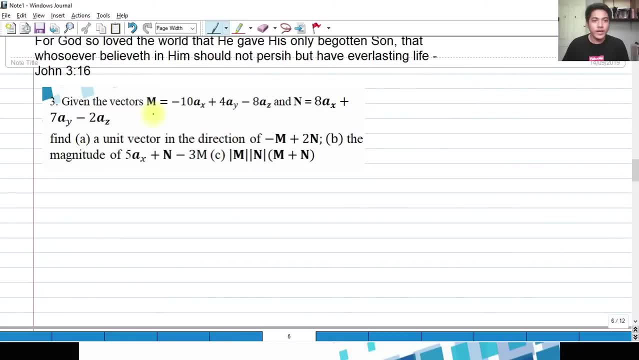 Okay, So moving on for our problem, let's say number 3.. Okay, Number 3,. given vectors m, negative 10ax plus 4ay minus 8az and n is equal to 8ax plus 7ay. 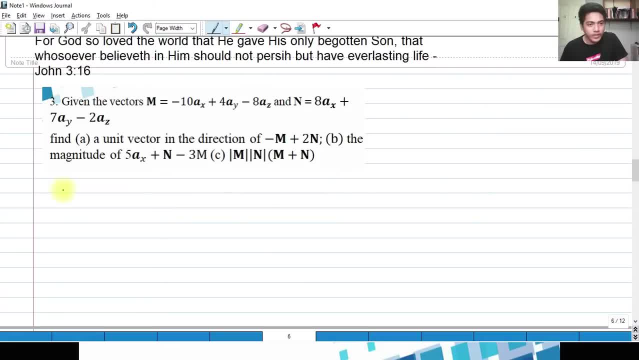 minus 2az. find letter a, the unit vector in the direction of negative m plus 2n. Unit vector, that is a, Okay, In the direction of negative m plus 2n. So first, before we can get the unit vector, of course we need to get negative m plus. 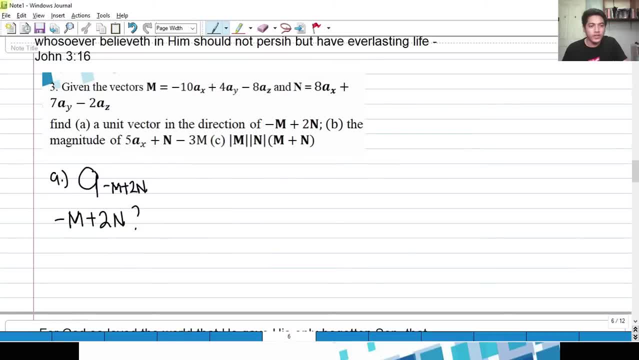 2n first. Okay, So let's try this. I will negate negative m vector negative m. So that would be negative. of the vector m which is negative, 10ax plus 4a sub y minus 8a sub z. 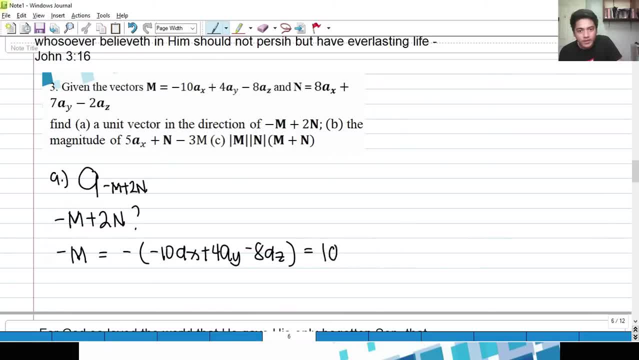 Okay, Distributing the negative sign, we have 10a sub x minus 4a sub y, plus 8a sub z. So this is our negative n. How about 2n? Twice the n. Okay, This is a scalar multiplied by a vector. 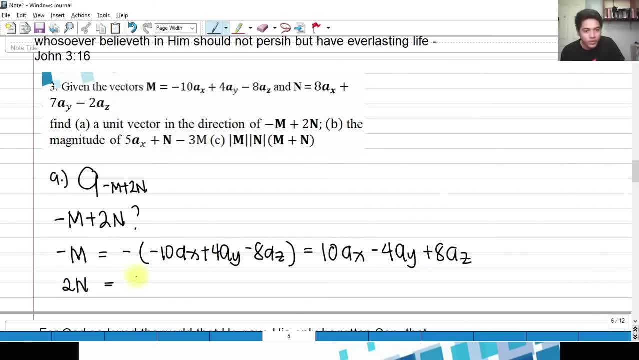 So scalar multiple of a vector. So we have twice the vector n, which is our. n is 8ax plus 7a sub y minus 2az, So we have 16a sub x plus 14a sub y minus 4a sub z. 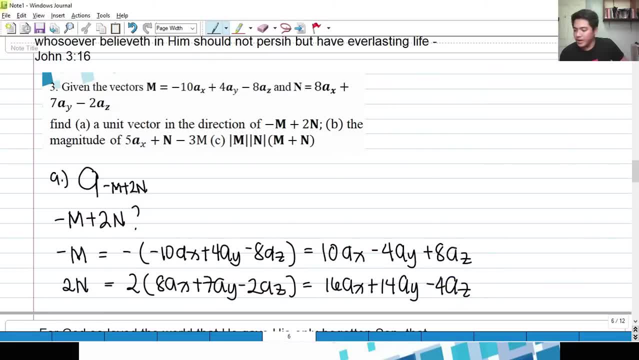 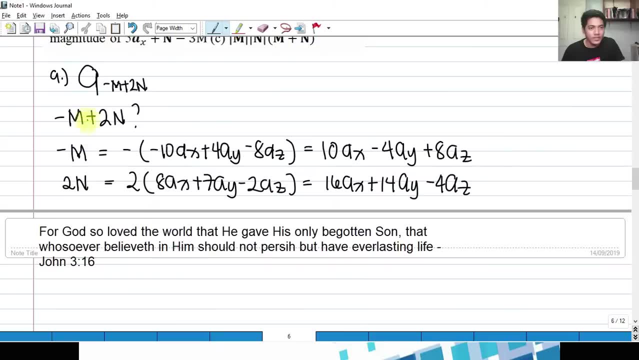 Okay, So that should be our twice of n. Okay, And if we're going to perform the vector algebra of this, negative m plus 2n, So negative m plus 2n, So we will add this: Okay. 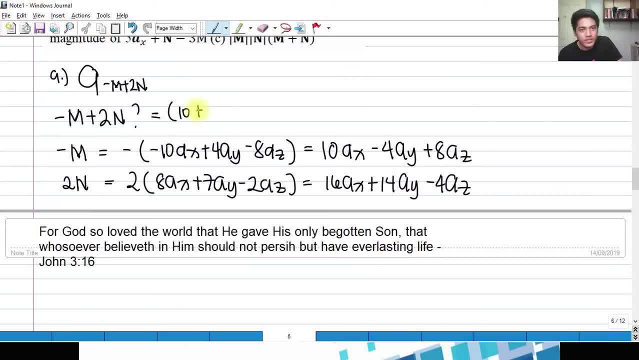 By components. So we have negative m, 10 plus 16a sub x plus negative 4.. This plus 14a sub y plus 8.. Okay, Plus negative 4, which becomes negative minus 4az. Hence our result shall be: 10 plus 16 is 26.. 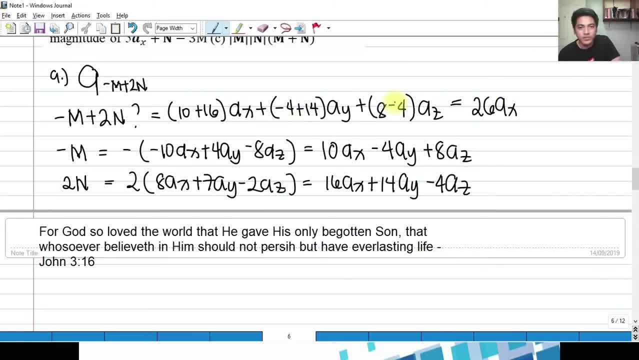 a sub x: negative. 4 plus 14 is plus 10a. sub y: Okay, Let me just rewrite this so that you would not be confused. ax, Okay, Oops, Let me try again. a sub x: Okay, And 6 plus 10 plus 4a. sub z: 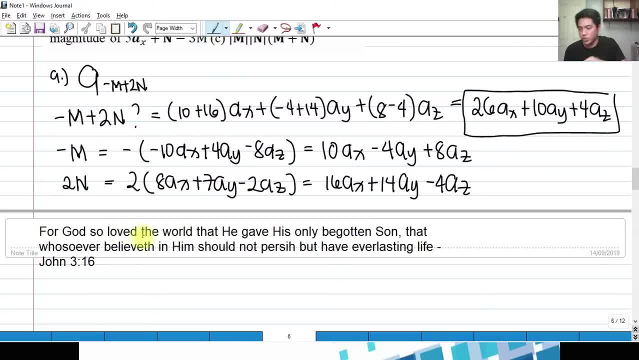 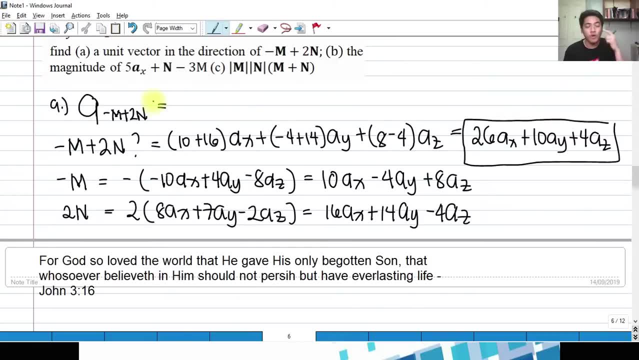 So this is our negative m plus 2n. Okay, Negative m plus 2n. That is not the final answer, because we are asked for the unit vector of negative m plus 2n, And the unit vector of negative m plus 2n is negative m plus 2n over the magnitude of. 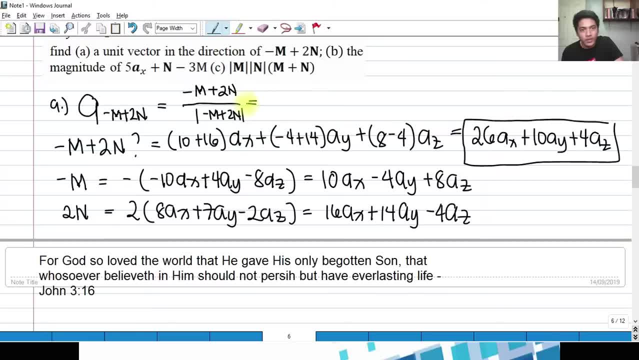 negative m plus 2n. And what is negative m plus 2n, That is 26a sub x plus 10a sub y plus 4a sub z. Over, okay, over. Let me just rewrite Over the square root of the components, which are 26 squared plus 10 squared plus 4 squared. 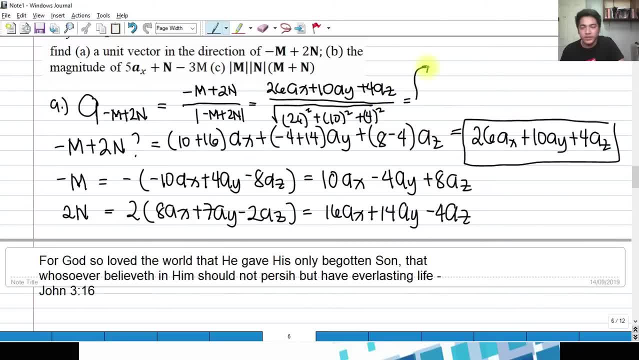 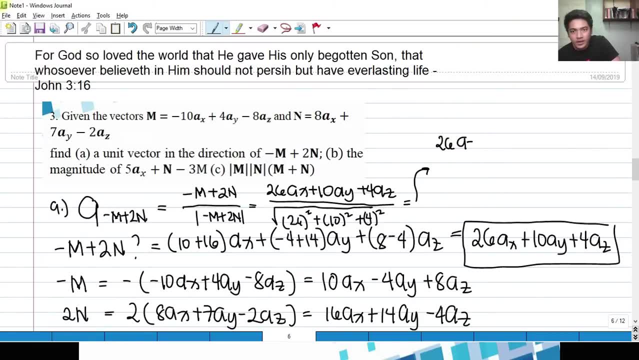 Okay, So let me have this the answer here. Okay. So how? Okay, Let's rewrite: 26a sub z over is a sub x plus 10 a y plus 4 a of z over, we have the square root of 6, square root of 22. so if you're. 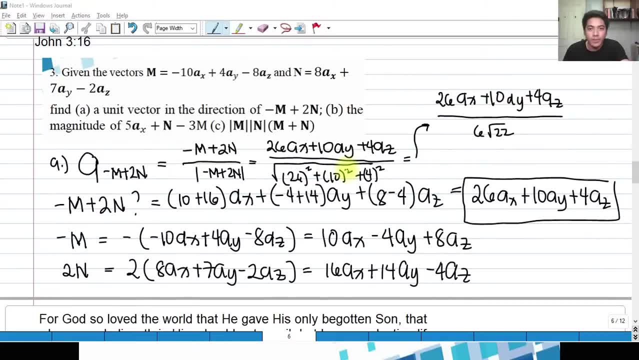 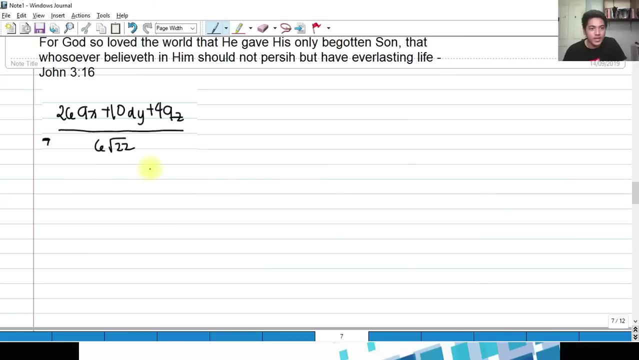 going to divide this all by components. i'm going to copy this first. okay, just give me time. i'm just just going to copy this to our here so that we can easily see. okay, so what happens is that when we have this, okay, by component, divide this plus 10 over 6, square root of 22 a sub y plus 4 over 6. 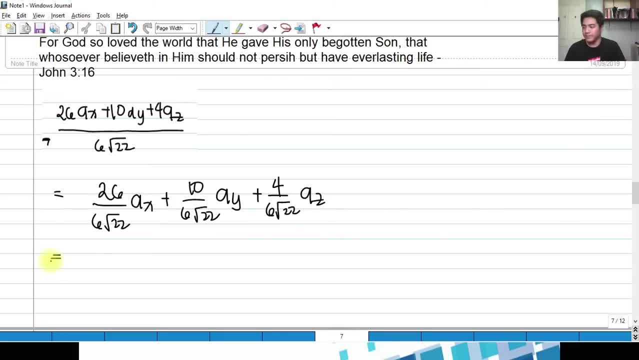 square root of 22 a sub z. you're going to evaluate it okay, by your calculator. so the result would be 0.92 a sub x plus 0.36- okay, a sub y plus 0.14 a sub z, which is the desired. 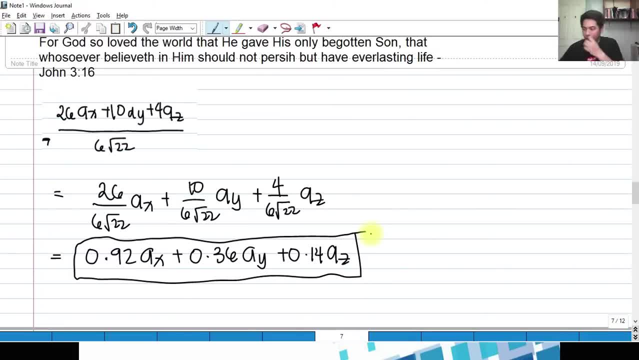 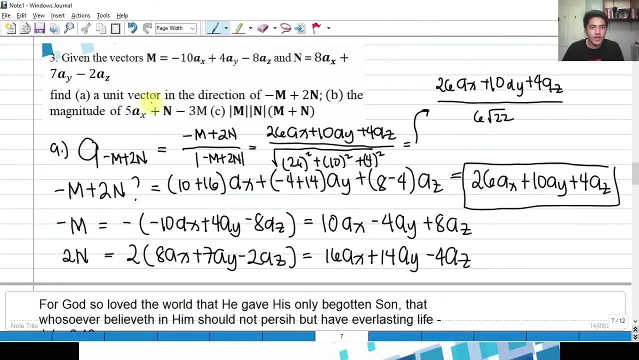 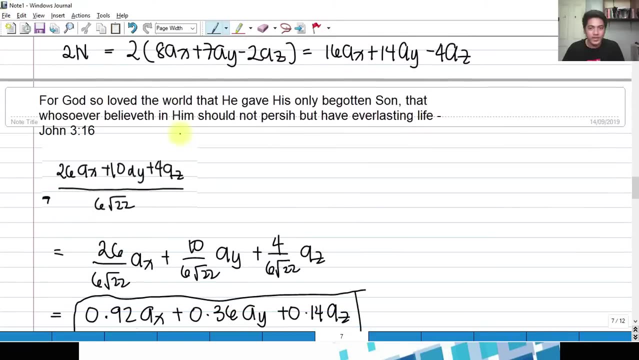 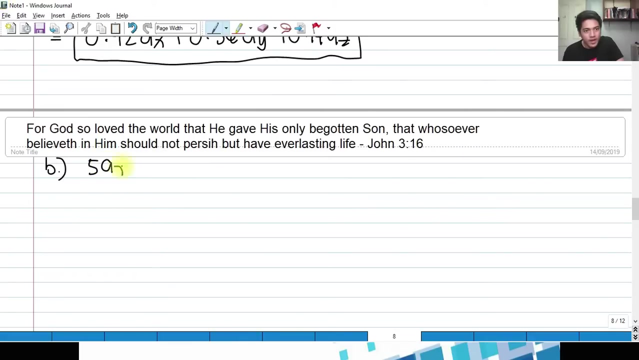 unit vector of negative m plus 2n. okay, so for letter b we shall be finding again the, what the magnitude of 5ax plus n minus 3m, 5ax plus m minus 3m, so the magnitude of the vector, 5ax magnitude. 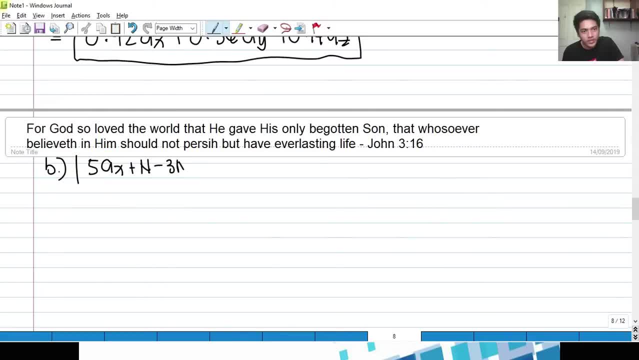 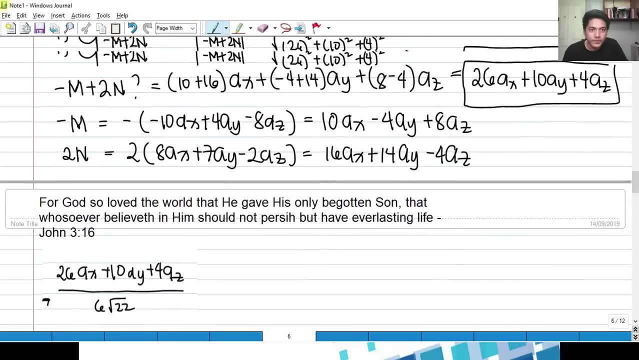 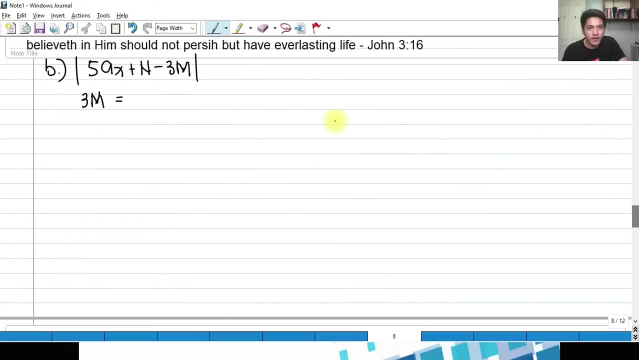 plus n, minus 3m, okay, so we don't have 3m, right, we don't have the 3m, okay. what is the 3m 3m thrice the vector m. so what is our vector m? negative 10, 4 and negative 8. negative 10, 4 and negative 8. no negative 10. 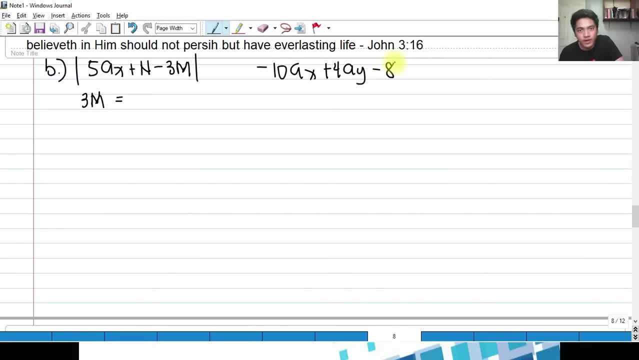 4 and negative 8 az. so what will happen? that should be 3 times negative 10 ax, plus 4 a sub y, minus 8 a sub z. so this corresponds to negative 30 a sub x. then we have plus 12 a y, minus 24 a z. okay, before a z. so this is only 3m if you apply negative 3m. 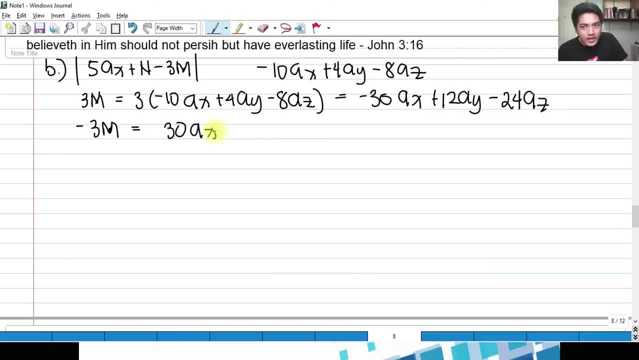 here, such that we negate this. this should be 30 ax plus or minus 12 a sub y, plus 24 a sub z. okay, why? because it has a negative here. so we're going to add this to all of, to all of the functions here, because to all of the vectors here, because we have distributed the negative sign, so we have. 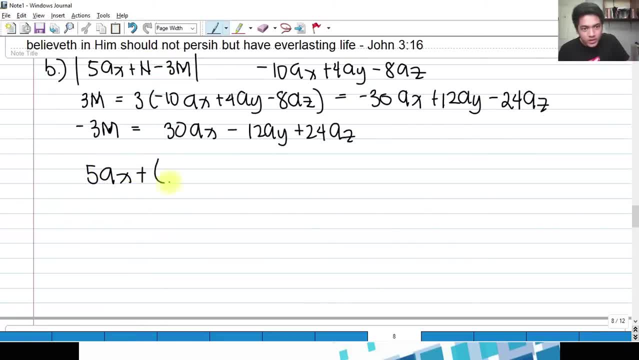 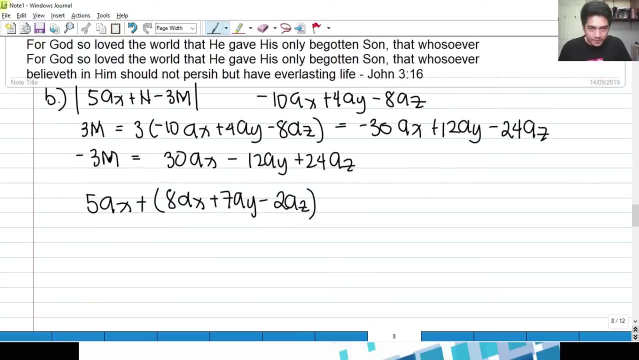 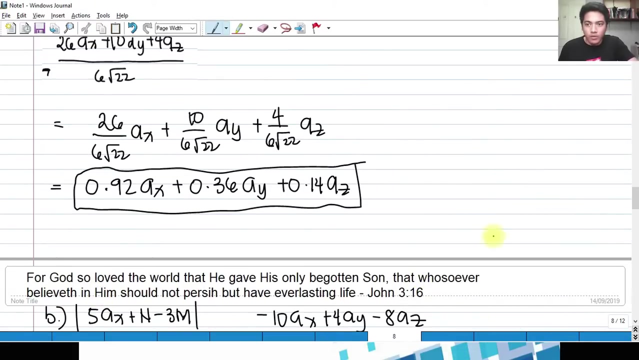 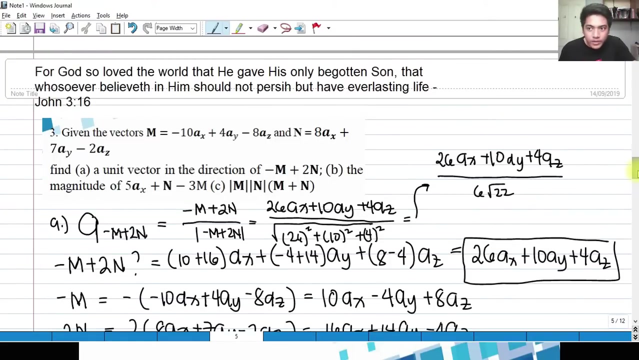 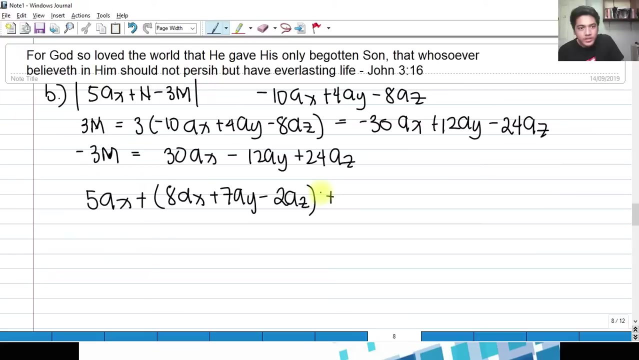 5ax plus what is our n? okay, our n is actually 8ax plus 7ay minus 2az. okay, let me check this out. just check it out. okay, if you have a correct value of, and here, 8, 7 and negative 2, okay, am i correct? 8, 7 and negative 2, okay, good to go plus, of course. 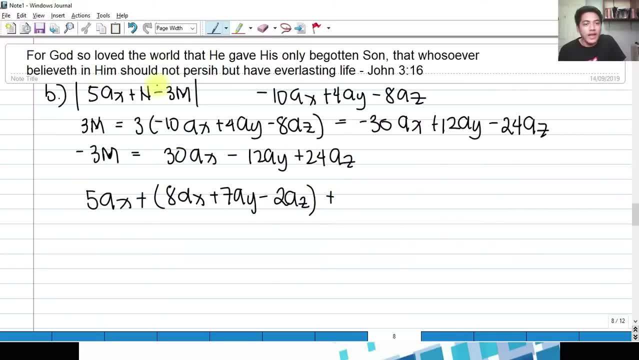 the negative 3m. okay, i plus it. i add it because i distributed already the negative sign, so to avoid confusion. so we have 30ax minus 12 ay plus 24 a z and this is the still the vector addition of these three, not still the vector addition. so if we have 5ax plus 8ax is 13ax. okay, plus 30, that should be 43. 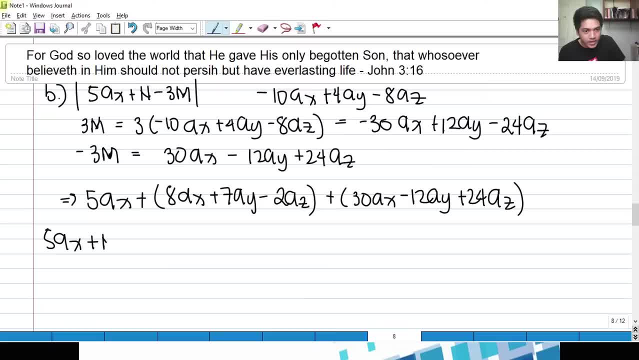 right, so 5ax. let's let me just rewrite: minus 3 is 5 plus 8. 13 plus 30, that is uh 43 a sub x ay 7. we have 7 ay minus 12. that is negative. what 5ay? if i'm not mistaken, then we have negative 2az plus 24. that should be plus 22 az. okay, that is. 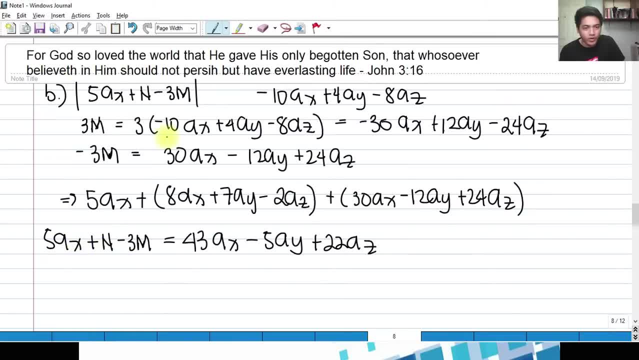 that is the 5ax plus n, minus 3m. perfect one, okay, if, in order for us to get the magnitude of this, okay, it's very easy. why? because we're going to get the sum of the squares of the components and then take the square root, so we 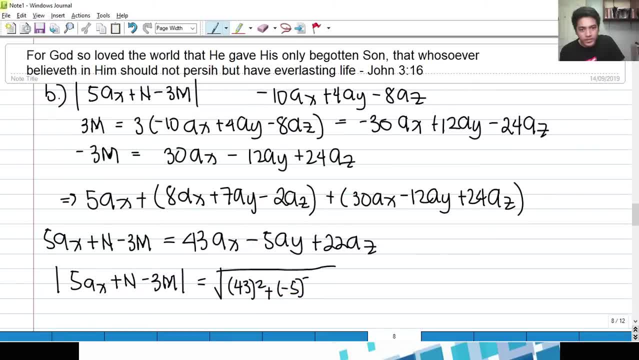 have 43 squared plus negative 5 squared, plus we have 22 squared and if you're going to calculate that, that should correspond to 48.6, and that is the magnitude of the square root. so we have the magnitude of this vector 5ax plus n minus 3m. okay, so that should be the answer. okay, so if we're 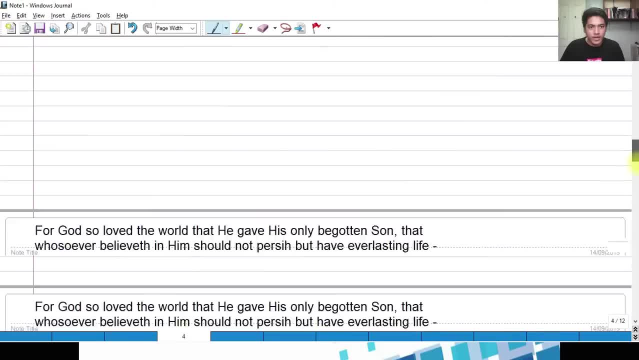 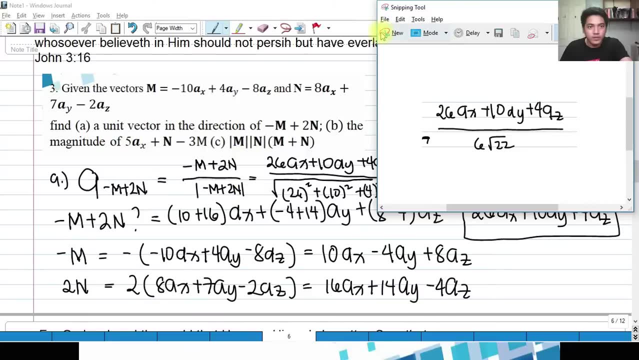 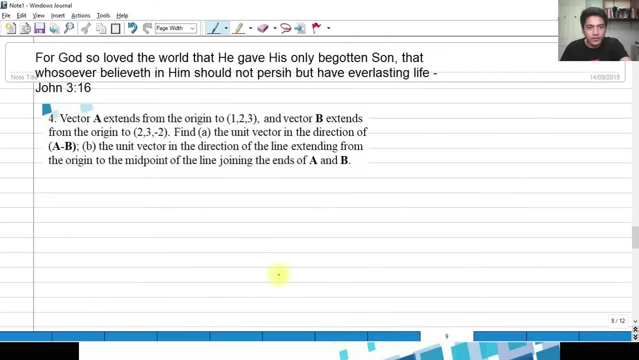 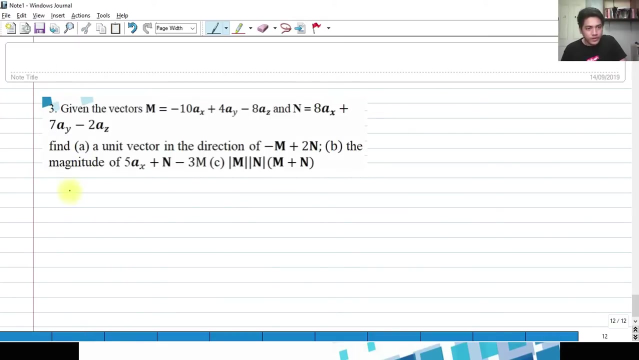 going to answer letter. let me just copy again the question. okay, copy again the question. going to copy the question? okay, and put it again. let's say on the other: so this would be our letter c. okay, letter c. so magnitude of m magnet times the magnitude of n multiplied by the m plus n vector. okay, we need to do first the magnitude, that's easy. 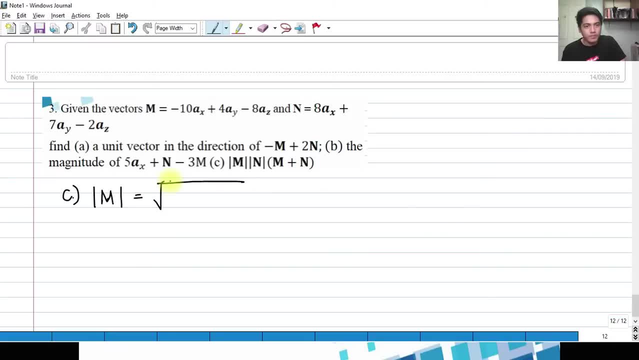 magnitude of vector m. we get the magnitude of vector m by negative 10 squared, okay, plus 4 squared root, plus negative 8 squared, okay. so if you get the magnitude of this uh m right here, okay, i think it's 6 squared of 5, if i'm not mistaken. okay, i'm not mistaken so. and then we get the magnitude of. 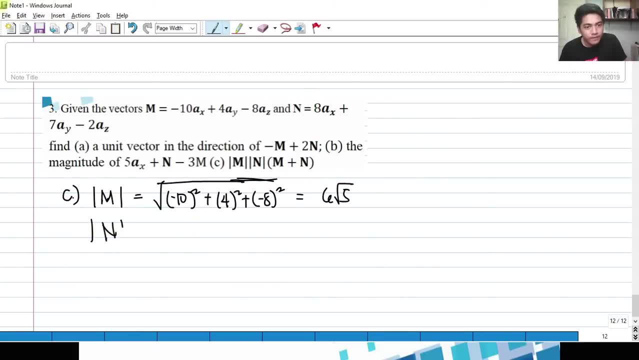 vector n: okay, we have square root of 2 squared plus 7 squared, plus negative 2 squared, and that corresponds to- let me just check it again: okay, so that corresponds to 3 square root of 13. okay, 3 square root of 13 we have. now. we have. 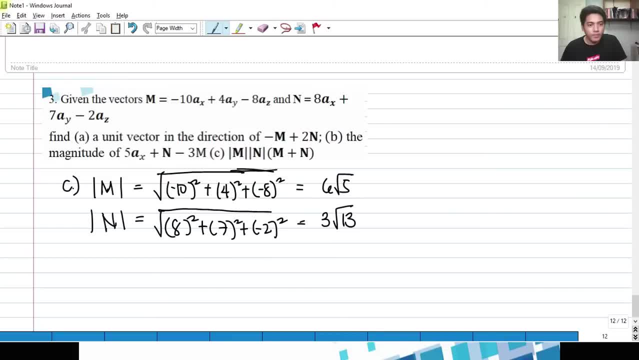 gotten now the magnitude m and n. okay, but we need to add m plus n. okay, if we need to add m plus n, so we have negative 10, okay, plus 8 a sub x plus okay, we have 4, and then plus 7 a sub y plus negative 8,. 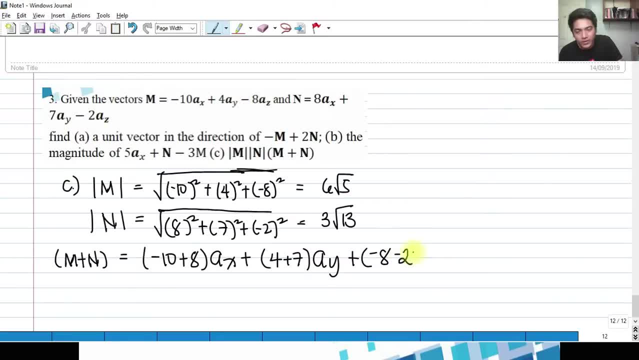 okay, negative 8 minus plus minus plus negative 2, so we have a j. so what will happen? we have negative 2, a x plus 11 a sub y minus 10 a sub j. okay, so again, it's simple if you perform this, 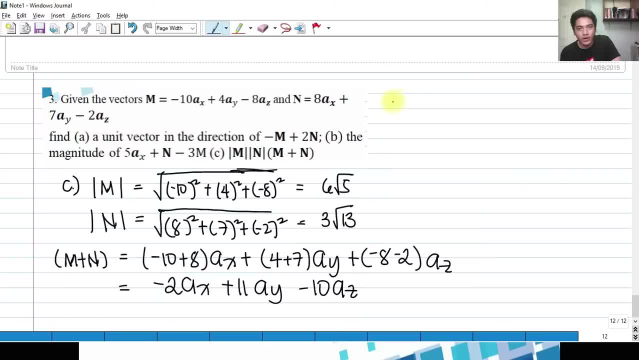 magnitude m times n. okay, what will happen? okay, so that should be 18 square root of 65,. okay, if you calculate it: 6,, 6 square root of of 5, multiplied by 3 square root of 13. let's check 18 square root of 65, okay, multiplied by the m plus. 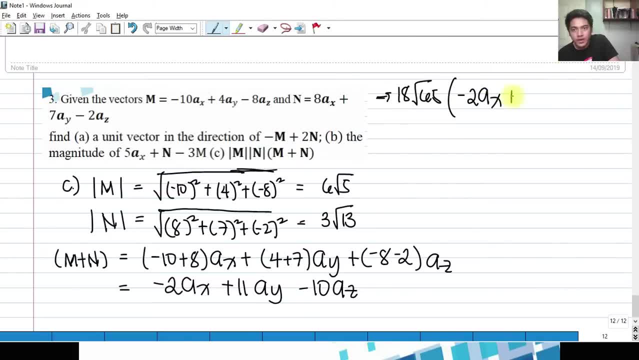 n, which is negative, 2 ax plus 11 a sub y, minus 10 a sub c. so if we multiply that, our answer should be negative. okay, 290 a sub x, plus we have 1596.33 a sub y. okay, 33, minus course, 1451.21. 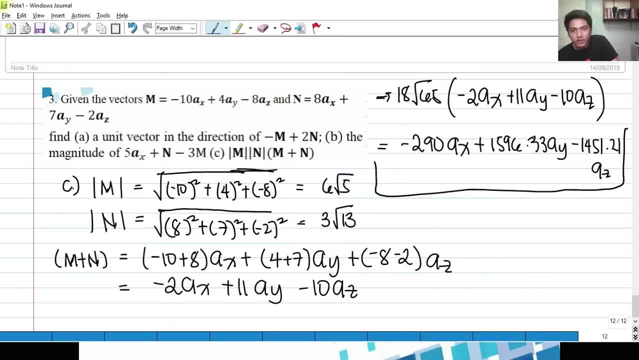 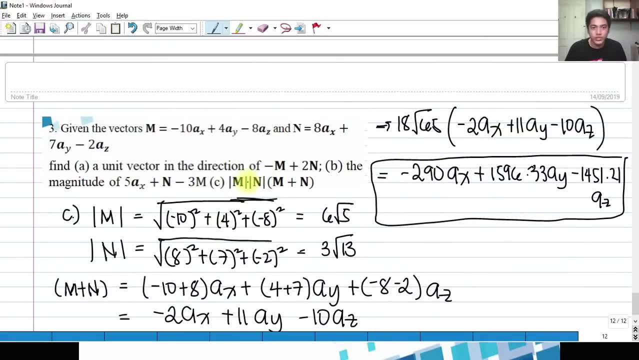 a sub c. so this should be our final answer. that is the vector we're looking for. remember, this is a magnitude times magnitude is scalar times scalar is scalar, but we multiply scalar by a vector, so our result must be a vector also, so hence, this is a vector. so this is our result for letter c. 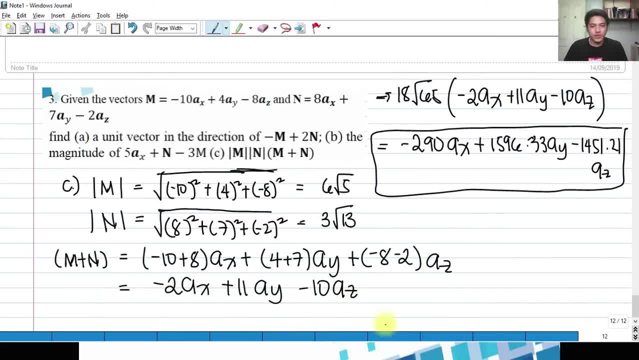 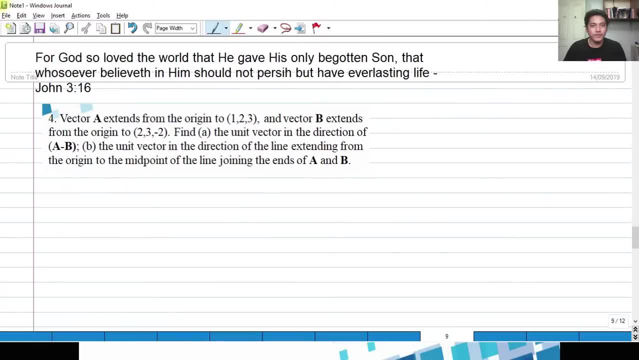 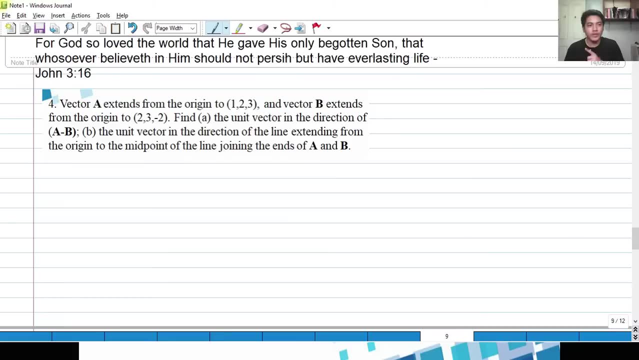 so let's go now to our very last number. okay, last question. okay, so we have, of course, uh, here, we have here. we have here: vector a extends from the origin to point one, two, three, and vector b extends from origin to two, three negative two find the unit vector in the direction of a minus b, so a minus b is a. 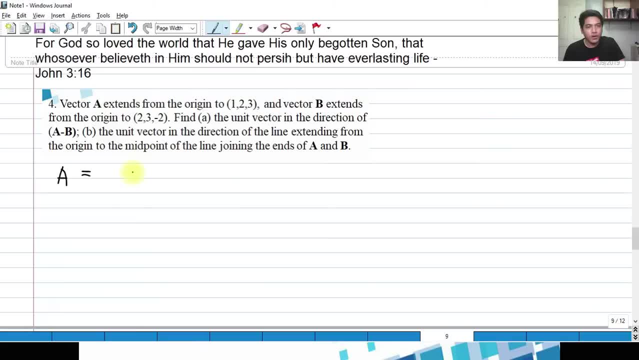 vector. so in order for us to get the vector a okay, we need to get okay from zero to origin, from origin to this point. that's the vector a. so one minus zero plus, or one minus zero a sub x. i'm so sorry, that's a vector, we're talking about vector. 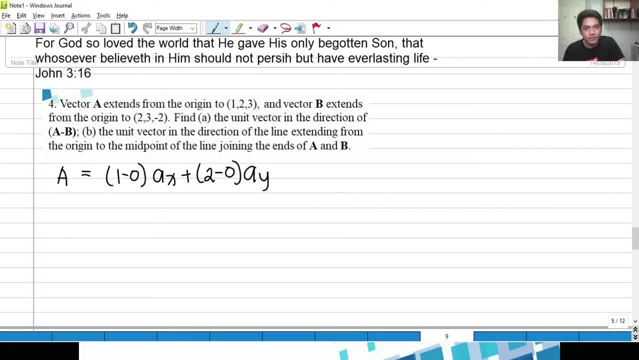 plus dash, plus A sub y. we need to find first the vector a and vector b. okay, so plus three minus zero. diagonally, this is A x plus two, A sub y, plus three a sub z vector and from vector b the same. okay, from origin to this point. 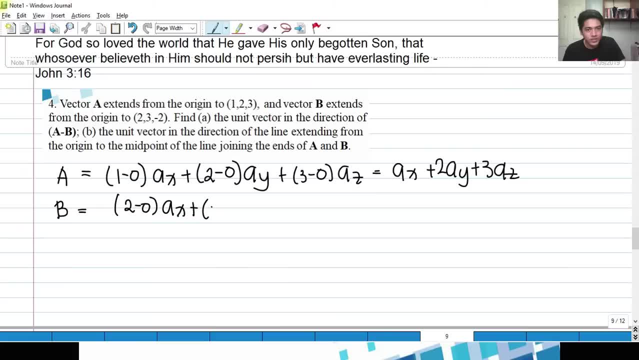 so two minus zero Max minus three minus zero a y plus negative. 2 minus 0 a sub z. so the result is 2 a x plus 3 a y minus 2 a z. it says the unit vector in the direction of a minus b. so a minus b would be okay. 1 minus 2 a x, okay. 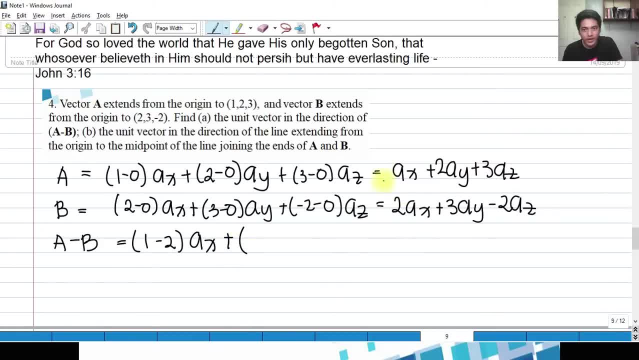 1 minus 2 a- x plus. okay. plus we have 2 minus 3 a- y. plus we have 3 minus negative 2 a sub z. okay, so we simply subtract a and b. okay? so what happened was that we have negative a- x minus. 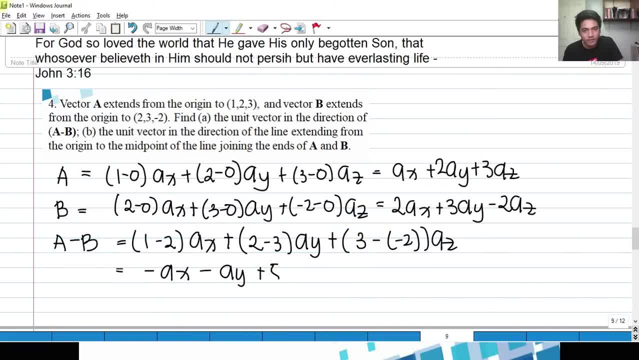 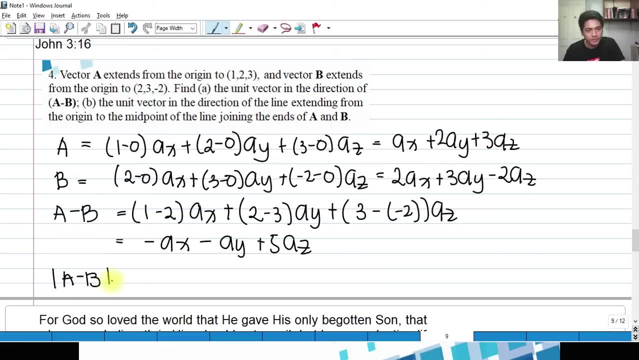 a, y, 3 minus negative 2 is plus 5 a- z right here. okay, so we now get the a minus b. so we are now get ready to get the magnitude of a minus b. okay, we have the square root of negative 1 squared plus negative 1 squared. 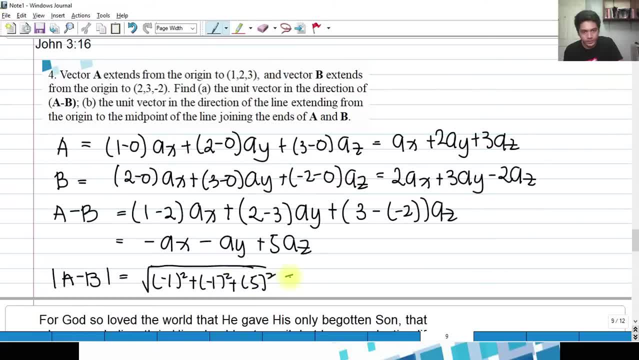 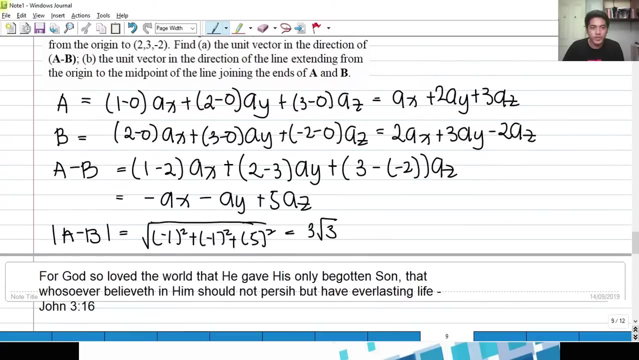 plus 5 squared, so that corresponds to a magnitude of magnitude of 3 squared of 3, if i'm not mistaken. so that if we're going to get the direction, okay, the unit vector, the unit vector in the direction of a minus b, we simply use the. 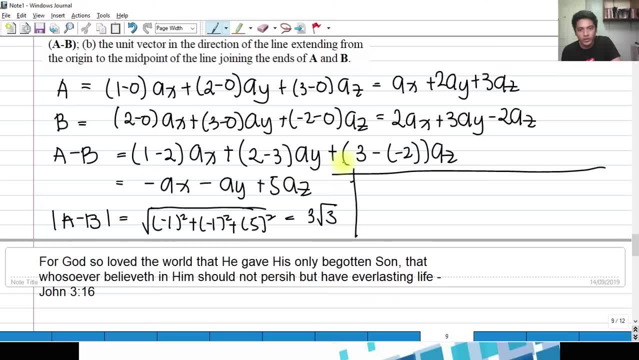 formula: okay, the unit vector is denoted by a of a minus b, is simply vector a minus b over the magnitude of a minus b. okay, the vector itself divided by its magnitude of which. we got it already. so a minus b is simply negative. a x minus a, y plus 5, a z over a minus b, the magnitude 3 squared of 3. so if 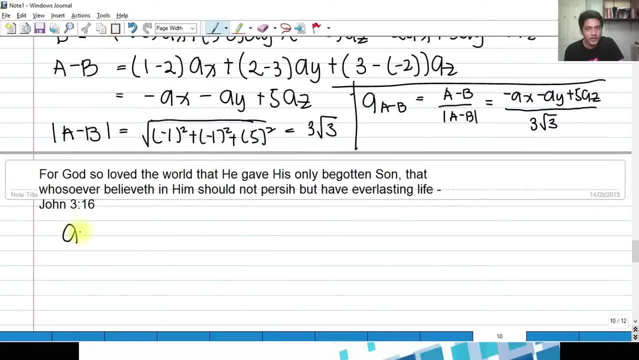 we're going to get that. what will happen is unit vector of a minus b is negative 1 over 3 squared. we have negative a v times a5 plus 4z. so that contrasted already. I already subtracted, talking to aIST, that we got the hacia- who's is negative a unfолжt. so we need. 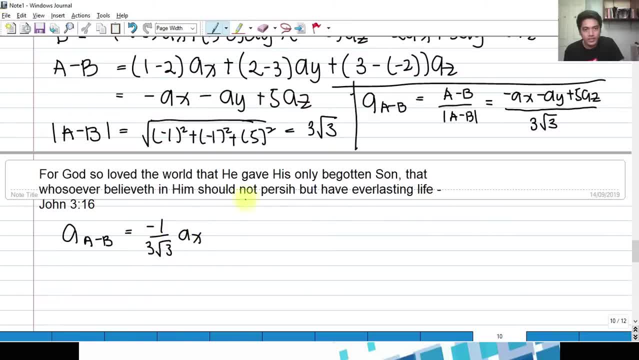 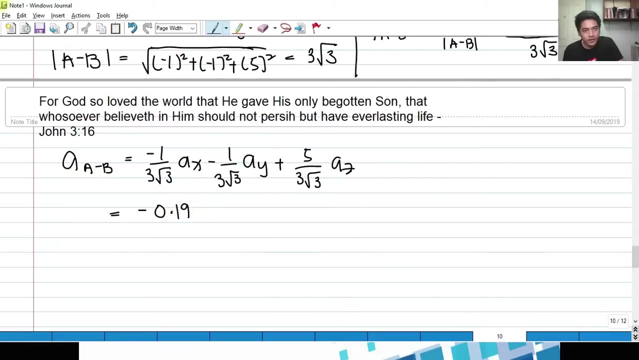 Negative: 1 over 3 squared of 3 AX minus 1 over 3 squared of 3 AY. We simply divide the coefficients of this by this Plus 5, 3 squared of 3 AJ, And if we're going to have it calculated by our calculator, that is simply negative: 0.19 A sub X minus 0.19.. 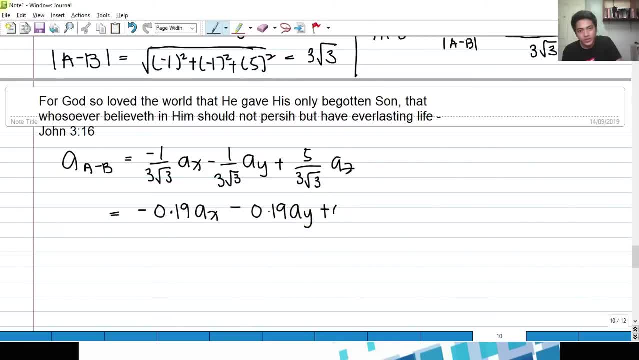 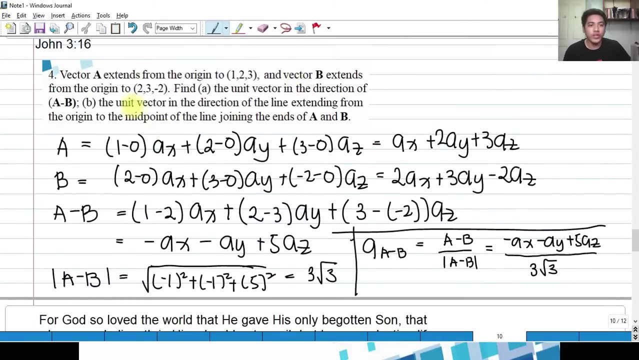 A sub Y, that is the same Plus 0.96 A sub Z. Now, this is the unit vector in the direction of A minus B. Okay, So for letter B, for our last example, the unit vector in the direction of the line extending from origin to the midpoints of the line joining the ends of A and B. 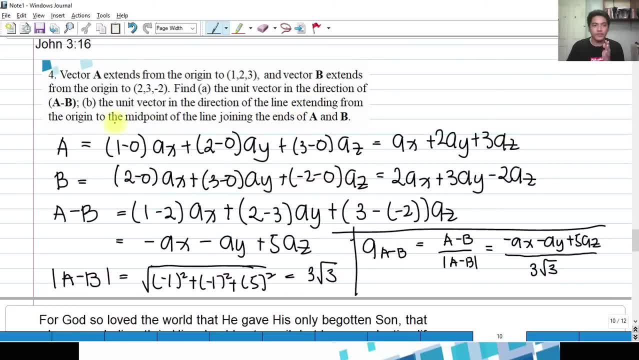 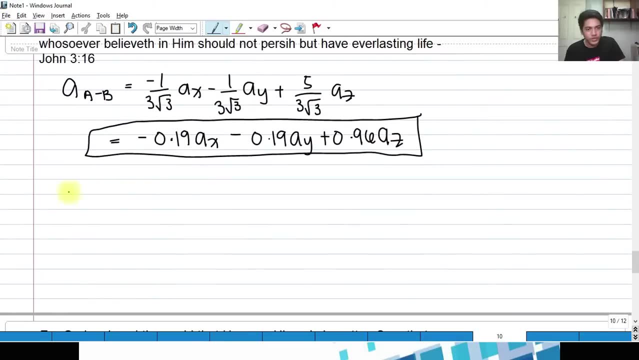 The unit vector in the direction of the line extending The unit vector in the direction of the line extending from the origin to the midpoint of these two points. Okay, So, joining the lines of the ends of A and B. So what are we going to do- is, first, we're going to find the midpoint of AB. 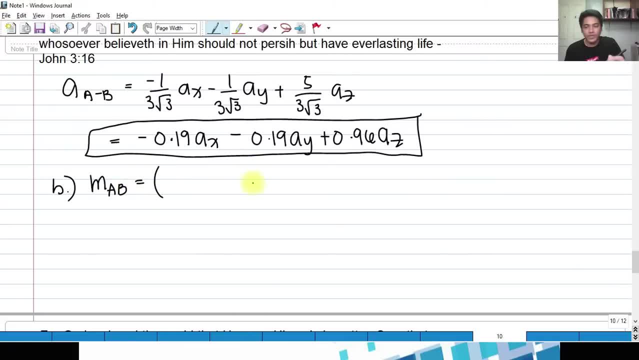 Okay, The midpoint of AB is given by X sub 1 plus X sub 2 over 2.. So in this case we have 1 plus 2 over 2, because X sub 1 is 1, X sub 2 is 2.. 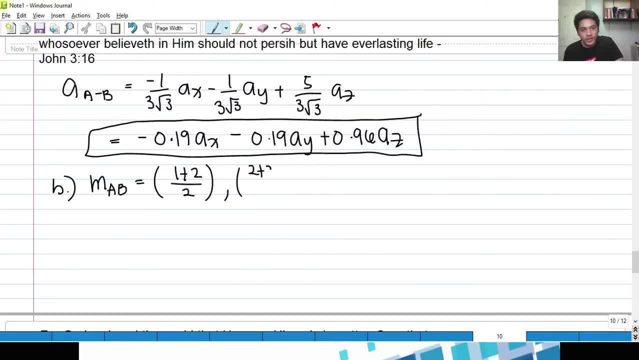 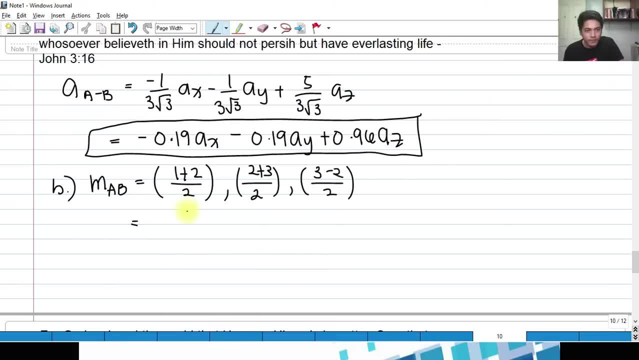 So for Z. So the XYZ midpoints are 3 halves. Okay, We have 2 or 5 halves, I'm not My mistake. 5 halves 3 plus 2. That is 5 halves, Okay. 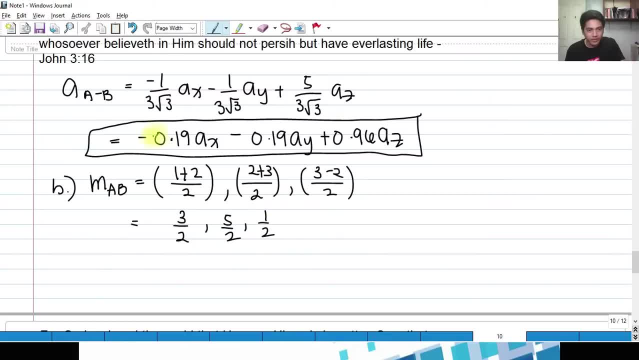 Then we have 1, half, so that is the midpoint of a and b. the problem is actually asking us: okay, okay, the, the, the unit vector of this vector that we're going to form from origin to this a, b, midpoint a, b, so to get the vector okay and emphasize the vector, this is only this, is only the, the, the points of the. 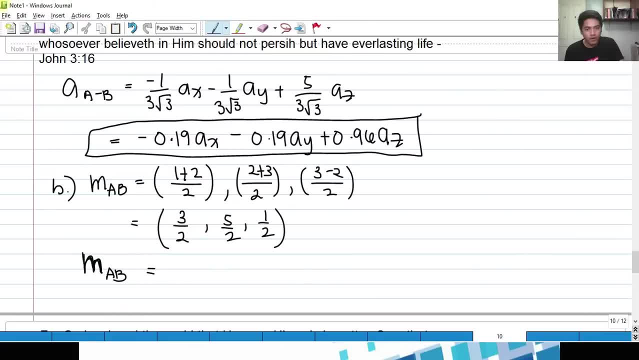 midpoints of the two points given. so we're going to get now from the origin. so this is the terminal point and the initial point is origin. so that's simply three halves minus zero a x plus five halves minus zero a y plus one half minus zero a j. so it only means that that is equal to 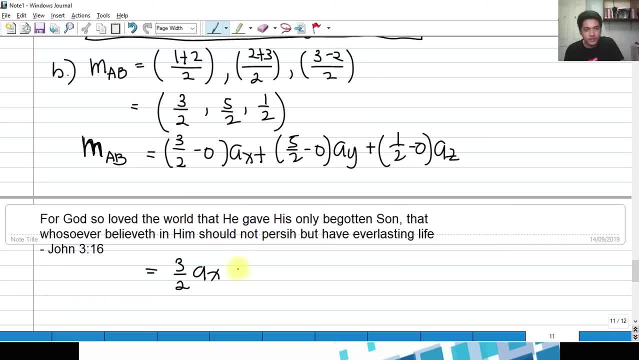 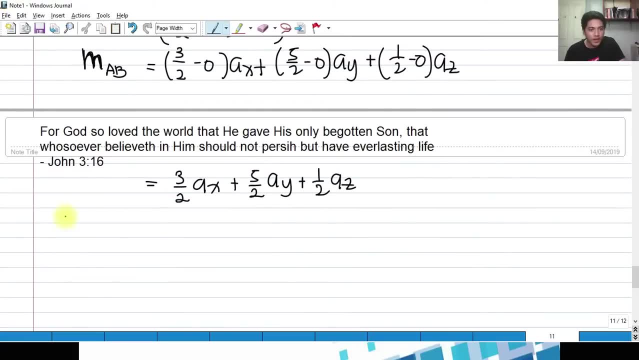 three halves a sub x plus five halves a sub y, so plus one half a sub j and we're going to get the unit vector in the direction of the midpoint of a and b. we have the vector of the midpoint of a and b over the magnitude of the midpoint of. 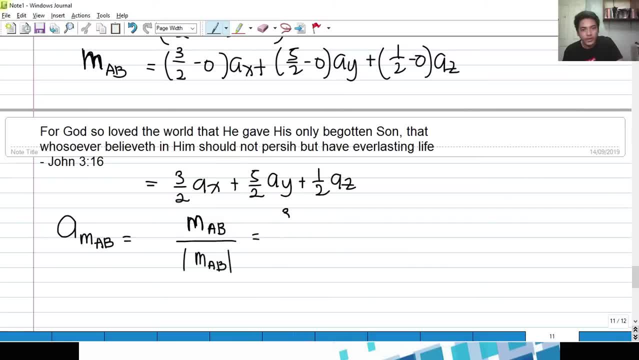 vector a, b. okay. so we have three halves a sub x plus five halves a sub y plus one half a sub j. okay, divided by the magnitude, okay. so i'm going to make this decimal: three halves is 1.5 squared 2.5. five halves is 2.5 squared plus one half 0.5 squared. so let's try, i'm going to make this. 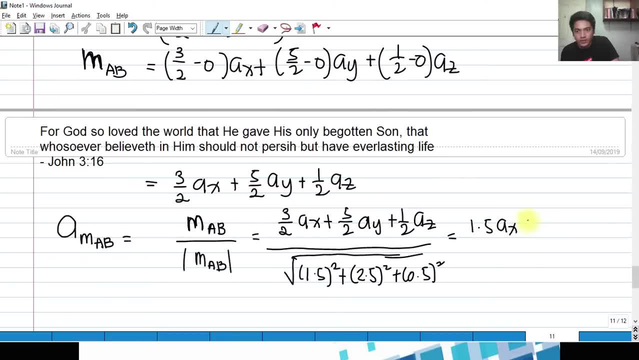 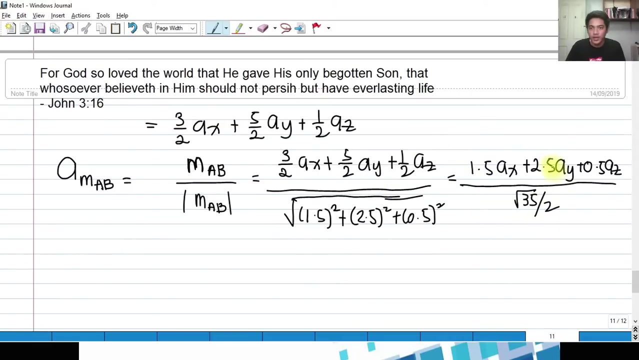 decimal. so 1.5 a x plus 2.5 a sub y plus 0.5 a sub j, divided by okay, divided by that square root. let me just first calculate it, okay. so we have square root of 35 over 2, square root of 35 over 2, and if again we divide this coefficient with this, okay, each. 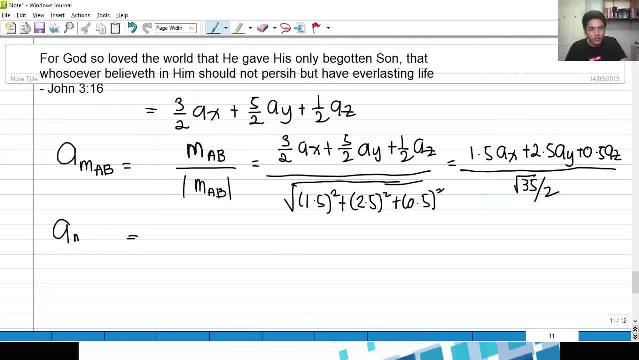 coefficient, we shall be arriving at an answer of the unit vector of the midpoints a and b. vector a, a and b. a and b, we have two 0.96. okay, a sub x, that is 1.5 divided by square root of 35 over 2 a x. that's the result, so plus. 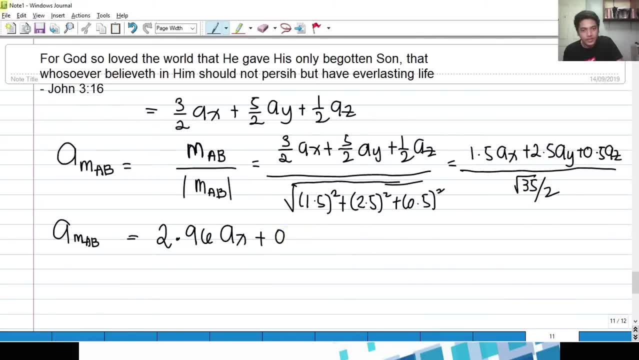 2.5 divided by square root of 35 over 2, that is 0.85 a sub y. and lastly, we have plus 0.8, 17 a sub z. so this is the unit vector of the midpoint joint the points a and b, the vector unit vector joining the points midpoint a and b. okay, so if you found, 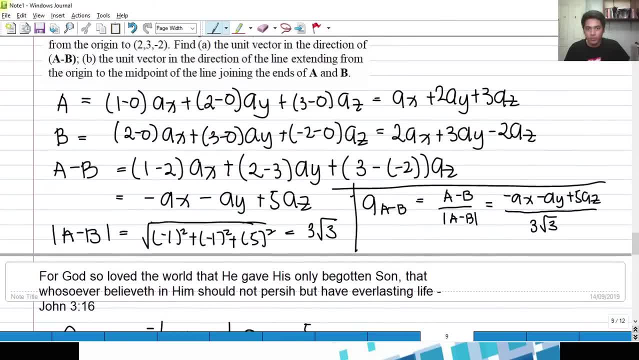 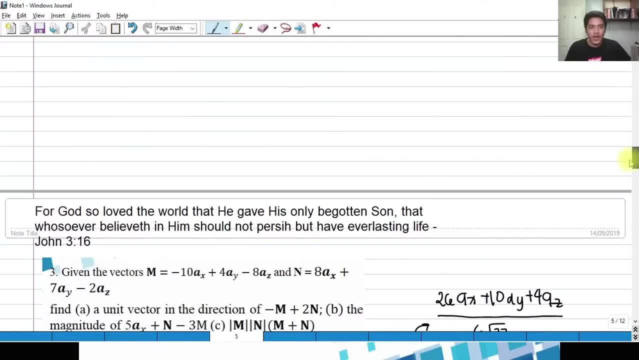 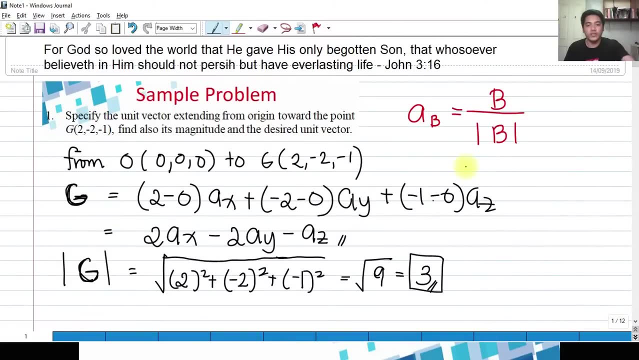 this video helpful. don't forget to subscribe. thank you so much for listening. this is a lengthy discussion, but i hope you learned something about the vector analysis today in electromagnetics. so thank you so much for listening. have a great day. god bless you.